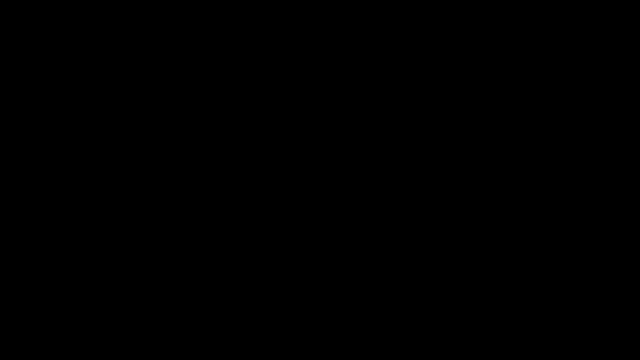 So, therefore, 5 plus 3 is 8.. Now, let's try this. Let's try this. Let's try some more examples. What is negative 4 plus 5?? Let's use the number line to get the answer. So we're going to start with negative 4, and we're going to add 5 to it. 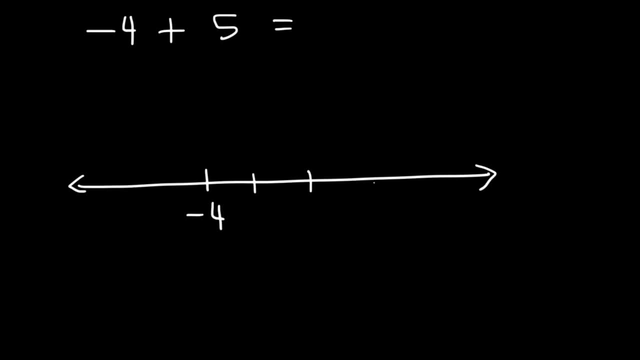 So we're going to travel 5 units to the right: 1, 2,, 3, 4, 5.. This is negative 3, negative 2, negative 1, 0, 1.. So negative 4 plus 5 is positive 1.. 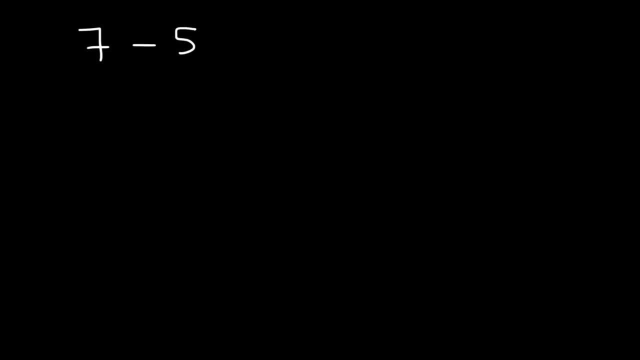 Let's work on another example: 7 minus 5.. So we're going to start with 7, and this time we're subtracting it by 5.. So we need to travel 5 units to the left: 1,, 2,, 3,, 4,, 5.. 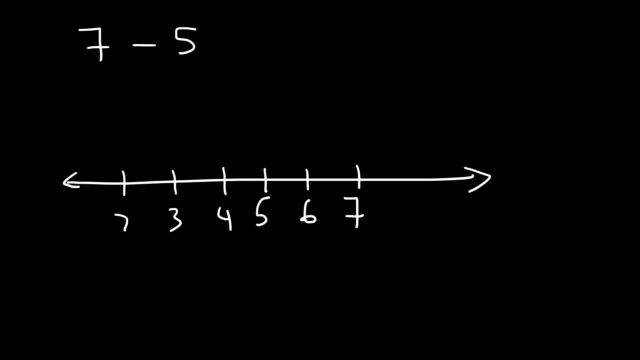 So this is 6, 5, 4, 3, 2.. So 7 minus 5 is 2.. Now, what about negative 4 minus 2?? So let's start with negative 4, and we're going to subtract it by 2.. 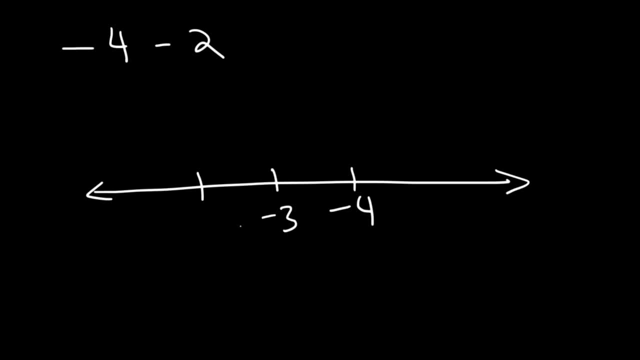 So we need to go 2 units to the left, And actually that should be negative 5.. Negative 3 is on the right side, So this is negative 6.. Therefore, negative 4 minus 2 is equal to negative 6.. 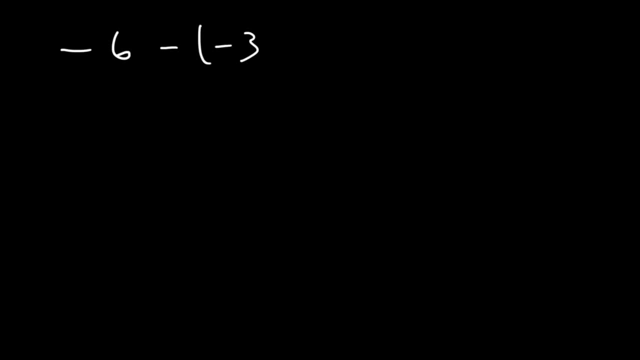 Now, what about this one Negative 6 minus negative 3. If you were to see something like this, you would see that this is negative 6.. If you were to see something that looks like that, what would you do Whenever you have two negative signs right next to each other? 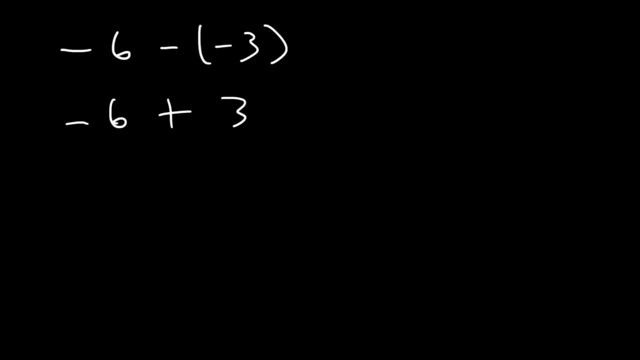 it's equivalent to a positive sign. When you multiply a negative by a negative, it's equal to a positive number. So we'll look at it for negative 6 plus 3.. So if we're adding, we need to travel to the right. 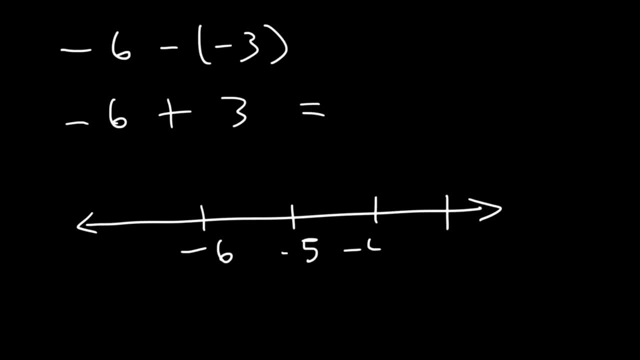 1, 2, 3.. This is negative 5, negative 4, negative 3.. And so negative 6 plus 3 is negative 3.. Now what about 8 plus negative 5?? What's the answer for this one? 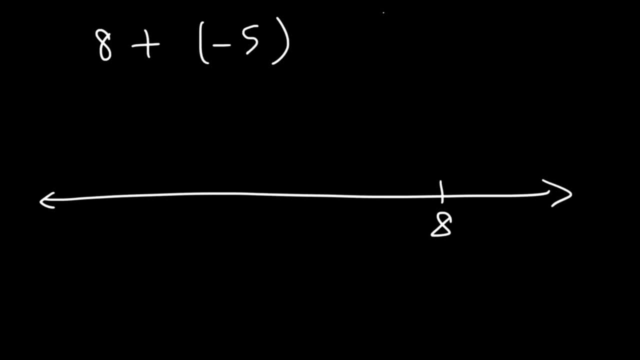 So if we start at 8 and we're subtracting it by 5.. By the way, this expression is equal to 8 minus 5.. A positive times a negative is a negative sign. So we need to travel 5 units to the left. 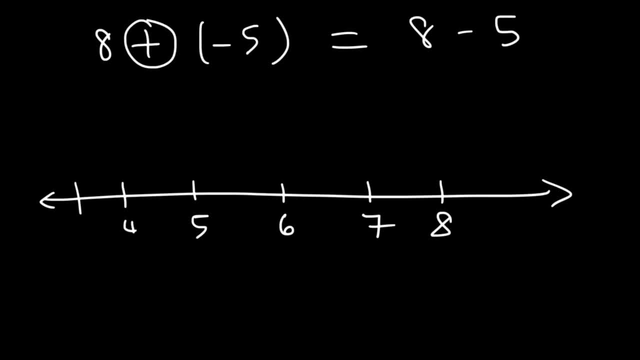 This is going to be 7, 6,, 5, 4, 3.. So 8 minus 5 is positive, Positive 3.. Now let's talk about multiplication. What is 8 times 3?? So you could answer this question easily if you have memorized your multiplication tables. 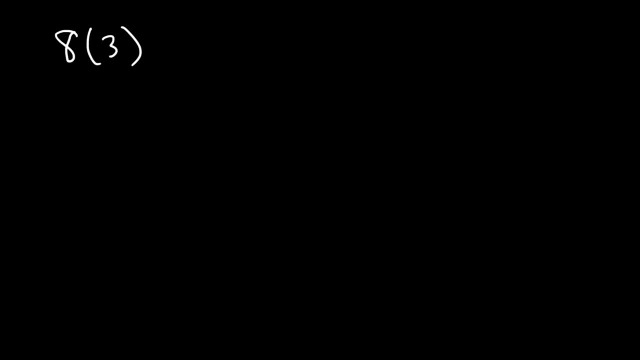 But in the event that you don't know, just remember: multiplication is simply repeated. addition 8 times 3 means that you're adding 8 three times. It's also equivalent to adding 3 eight times, But it's easier to add 8 three times. 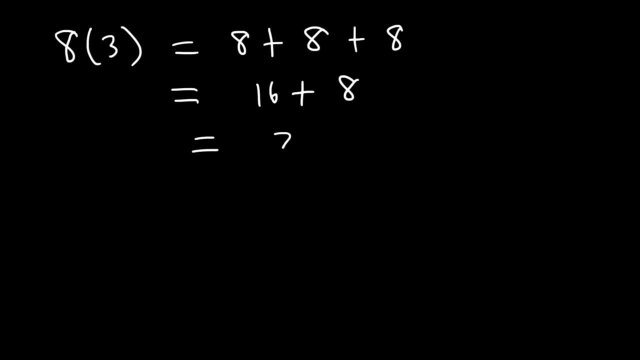 8 plus 8 is 16. And 16 plus 8 is 24.. So therefore, 8 times 3 is 24.. Let's work on another example. What's 9 times 4?? 9 times 4 is equivalent to adding 9 four times. 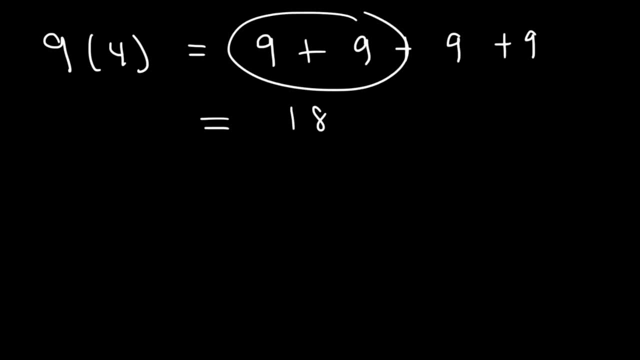 9 plus 9 is 18.. So these two 9s add up to 18.. And the other two 9s add up to 18 as well, And 18 plus 8.. 18 is 36.. So therefore, 9 times 4 is 36.. 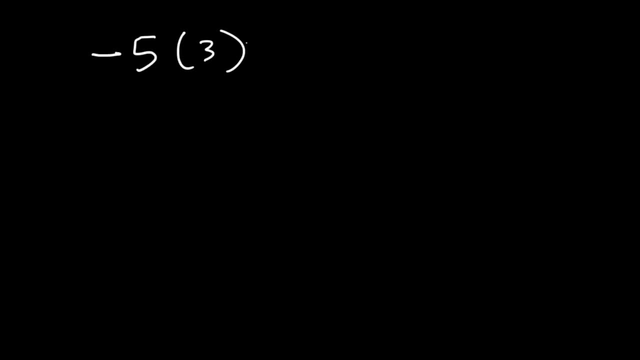 Now, what is negative 5 multiplied by 3? A negative times a positive number will give you a negative result, So we could just focus on adding 5 three times and then make the entire thing negative. 5 plus 5 is 10.. 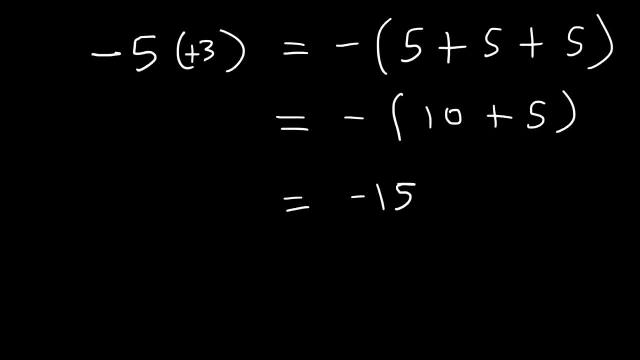 And 10 plus 5 is 15.. So therefore, negative 5 times 3 is negative 15.. Try this one. What is negative 6 multiplied by negative 8?? When you multiply two negative numbers, you're going to get a positive result. 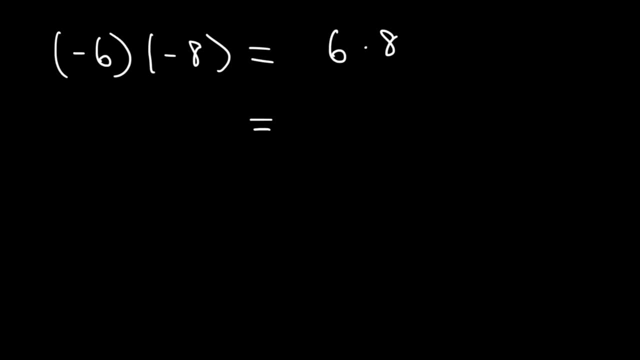 So this is equivalent to multiplying 6 times 8.. So I'm going to add 8 six times instead of adding 6 eight times. Now, adding two 8s is equivalent to multiplying 6 times 8.. Adding two 8s will give me 16.. 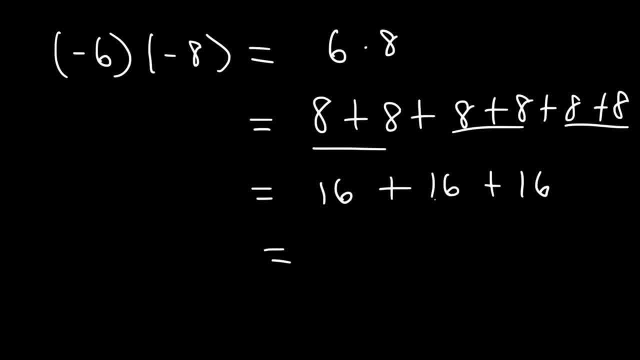 So I have 16 plus 16 plus 16.. And 16 plus 16 is 32.. And 32 plus 16 is 48.. So therefore, negative 6 times negative 8 is equal to this number, positive 48.. 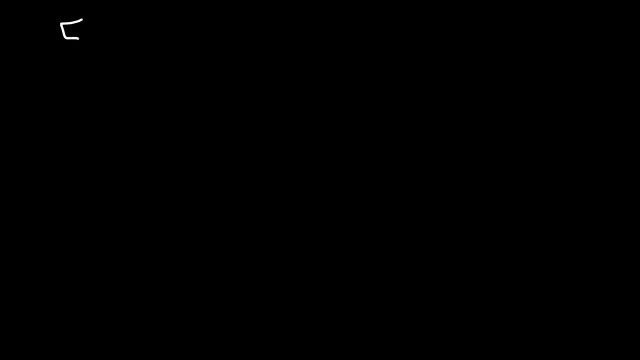 Now let's move on to our next example. Let's focus on division. What is 54 divided by 6?? Now it's important to understand that division is the opposite of multiplication. Six multiplied by what number is equal to 54?. 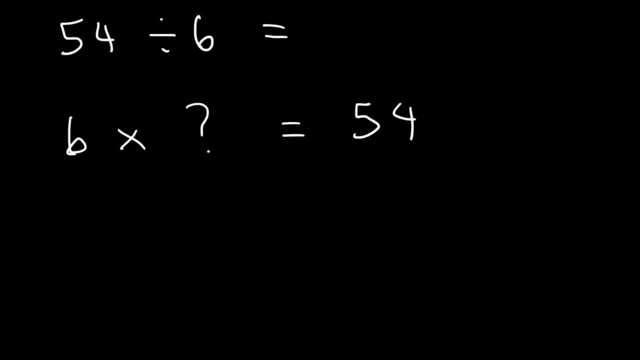 So how many times do you have to add 6 to get to 54?? It turns out that 6 times 9 is 54. So 54 divided by 6 is 9.. So division is simply the opposite of multiplication, Okay. 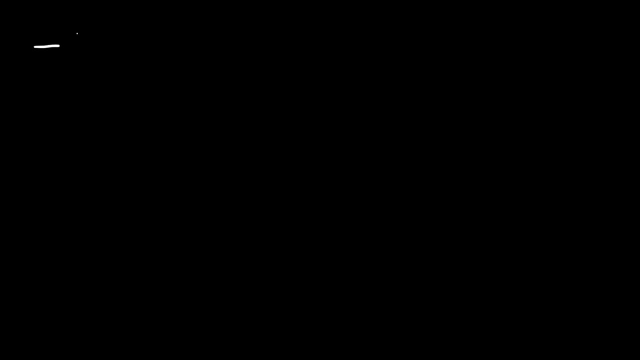 So here's another example: What is negative? 45 divided by positive 9?? A negative number divided by a positive number will give you a negative result. So we know the overall answer is negative. So let's just focus on dividing 45 by 9.. 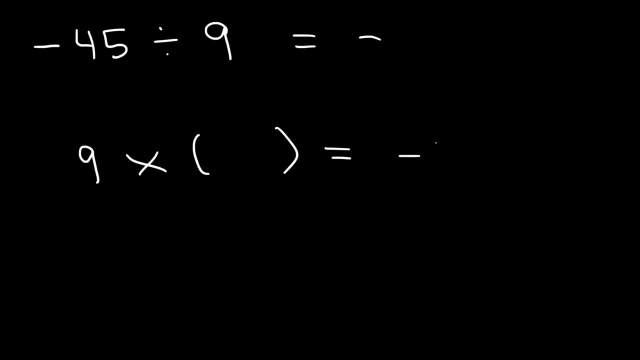 So 9 times what number is equal to negative 45? It turns out that you have to add 9 five times. You have to add 9 five times to get to 45.. Nine plus 9 is 18.. Eighteen plus 9 is 27.. 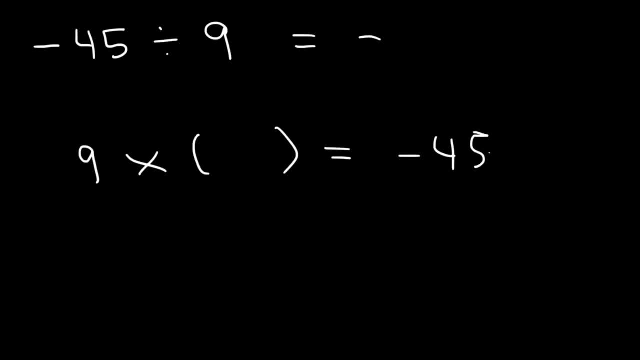 Twenty-seven plus 9 is 36.. Thirty-six plus 9 is 45. So therefore, 9 times negative 5 is negative 45. And if we focus on a reverse statement- negative 45 divided by 9, that's going to be negative. 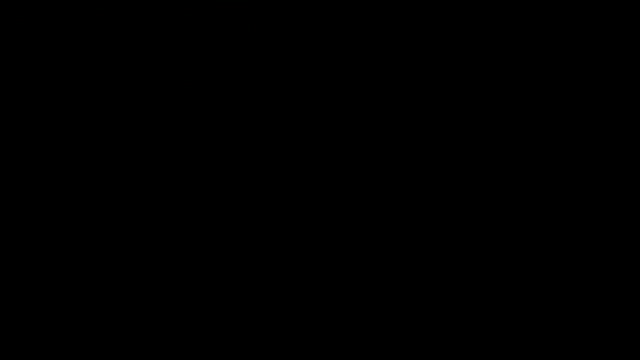 5. And so that's a quick and simple way to perform subtracting. It's as simple as that, Thank you. simple division. Here's another example: What's negative 12 divided by negative 2?? When you divide two negative numbers, you're going to get a positive result, So this is equivalent. 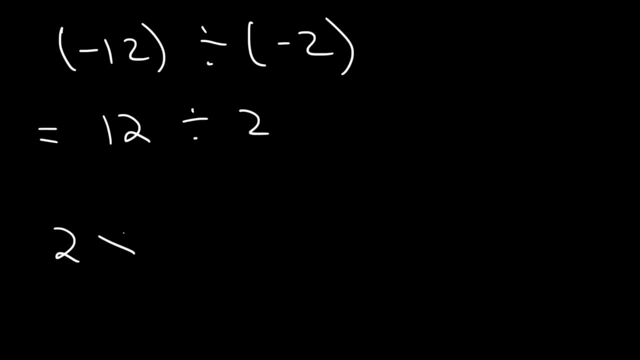 to dividing 12 by 2.. So 2 times what number is 12?? You have to add 2 six times to get to 12.. 2 plus 2 is 4.. If you add another 2,, that's 6, and then 8, and then 10, and then. 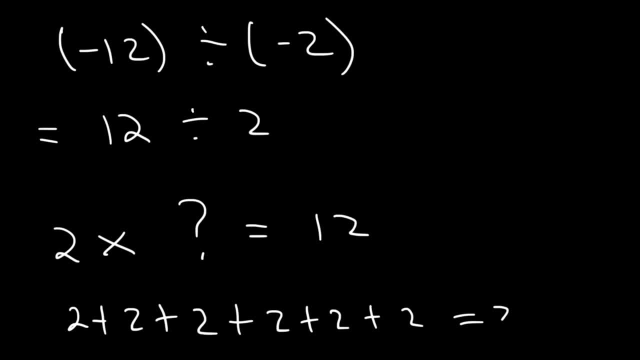 12.. So, therefore, 2 times 6 is equal to 12, and 12 divided by 2 has to be 6.. Now let's say, if you have this problem, What is 8 minus 5 times 4?? So what is the answer? Now, there's. 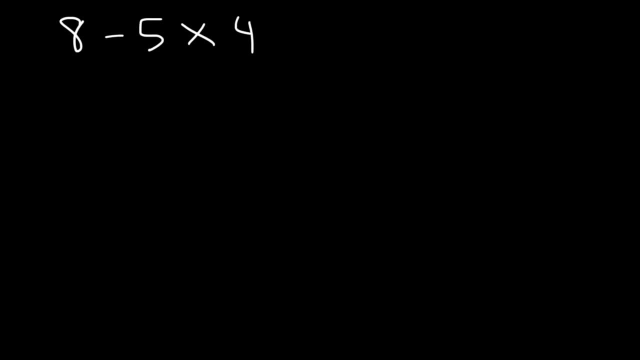 two possible ways of attempting to do this problem, And one of the two ways I'm going to show you is the right answer. The other is not. So should we subtract first or should we multiply first? If we subtract 8 minus 5, 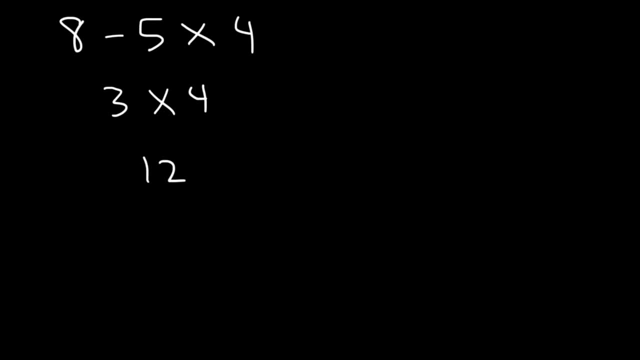 is 3, and 3 times 4 is 12.. We're going to get that result. But now let's say: if we multiply first Negative 5 times 4 is negative 20.. So this becomes 8 minus 20, and 8 minus. 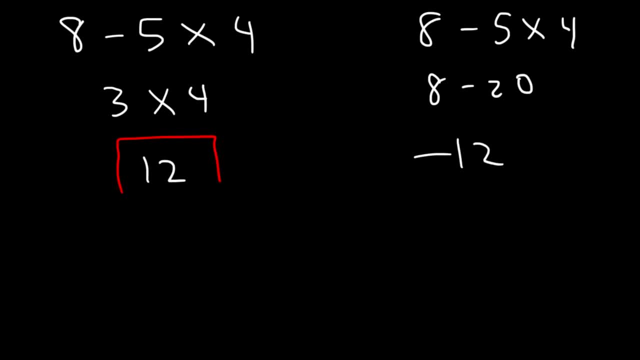 20 is negative 12. So the results are different. So which one comes first, Subtraction or multiplication? Perhaps you've heard of PEMDAS, Please excuse my dear Aunt Sally. P stands for parentheses E, exponents, M, multiplication, D, division. 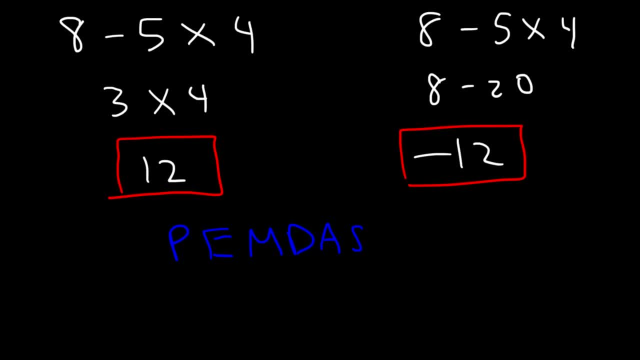 A is addition, S is subtraction, And so anytime you need to figure out which operation comes first, look at this expression. This is associated with the order of operations, And parentheses have the highest priority. Now we're comparing multiplication and subtraction, So therefore you should always multiply first before you subtract. Multiplication has more. 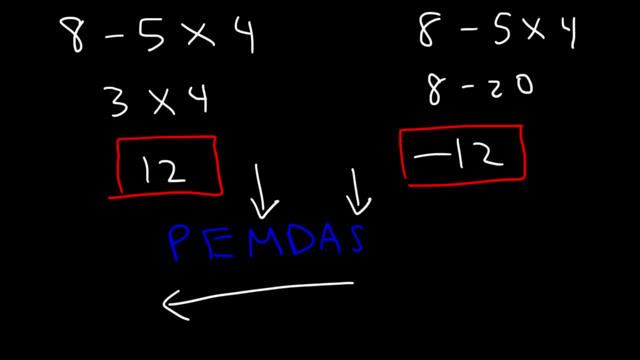 priority than subtraction. So that's how you can use PEMDAS to know which operation comes first. So therefore, this is the correct answer: 8 minus 5 times 4 is negative 12.. Now you can confirm your answer using a scientific calculator, if you have access to it. Simply 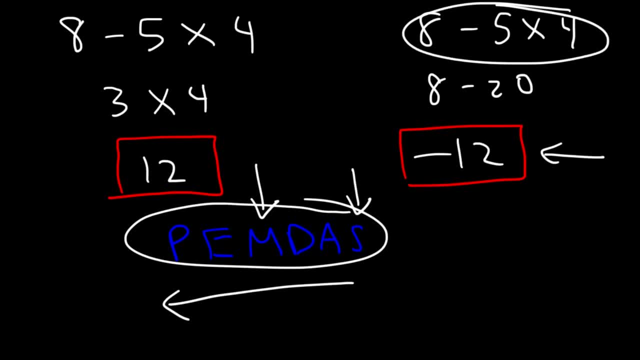 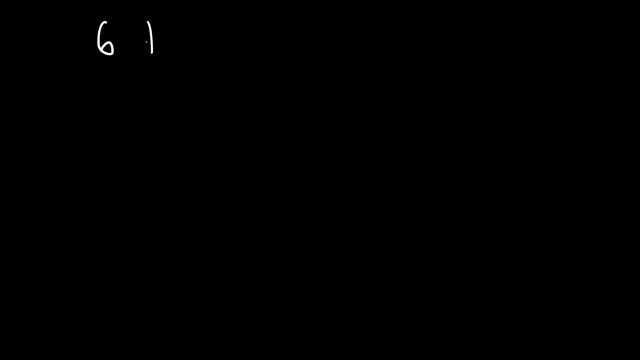 type this expression, exactly the way you see it, and the answer that you should get is negative: 12.. Now let's move on to another example. Try this one: 6 plus 24 divided by 4.. So feel free to take a minute and work on this example. So, according to PEMDAS, division has more priority over addition. 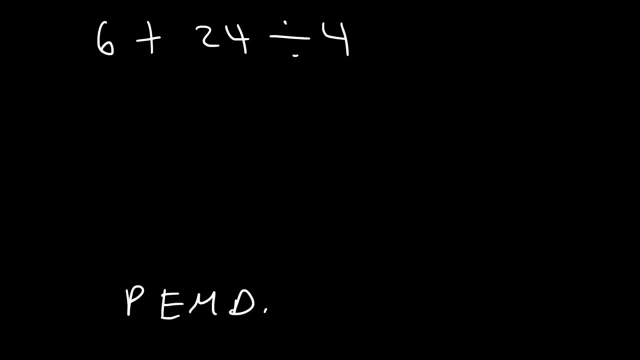 So P-E-M-D-A-S. So as you look at the letters towards the left, they have more priority over the letters on the right. So D is to the left of A. So division has more priority than addition. So you should divide first before you add. 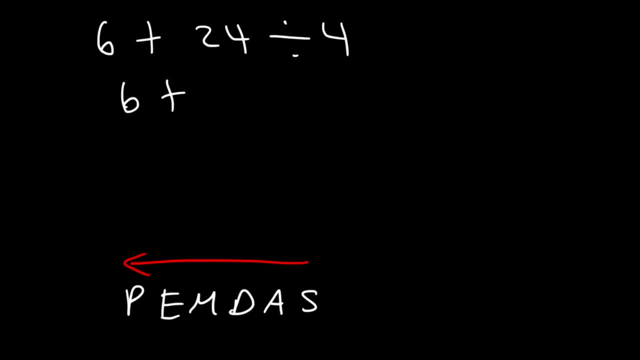 So what is 24 divided by 4?? 24 divided by 4 is 6, because 4 times 6 is 24.. And 6 plus 6 is 12.. So that's the final answer in this example. Now let's try another one: What is 8 minus 5 multiplied by 7?? 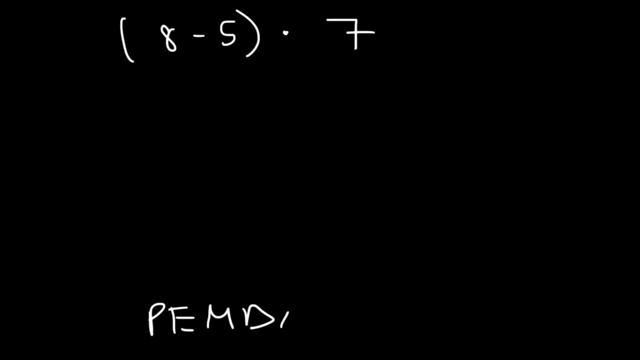 So should we subtract or should we multiply first in this case? In this case you should subtract, You need to perform the operation inside the parentheses, So you compare in parentheses to multiplication And you need to work inside the parentheses before you multiply. 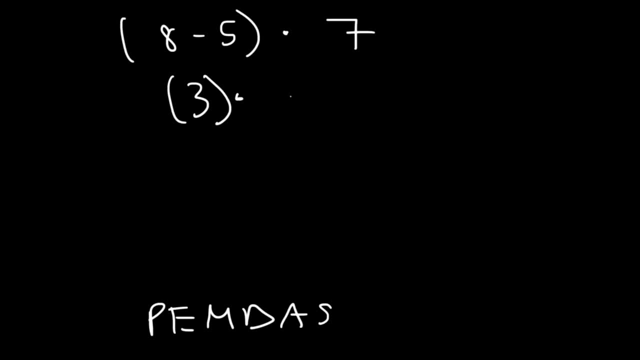 So 8 minus 5 is 3. And 3 times 7 is 21.. So that's the answer in this particular example. Now, what about this problem? What is 24 divided by 4 multiplied by 3?? Should we perform division first or multiplication? 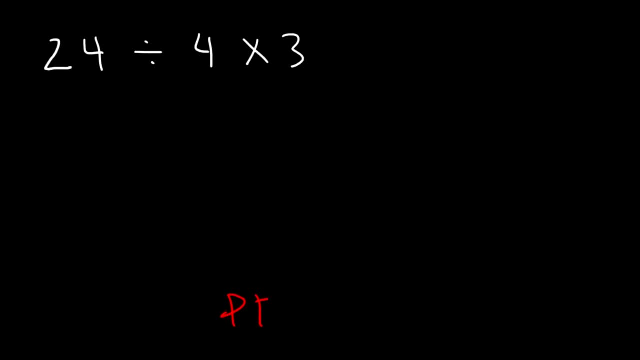 Now, according to the word PEMDAS, it appears that multiplication has more priority than division because it's on the left, But it turns out that these two terms are the same. These two terms, multiplication and division, they have the same priority. 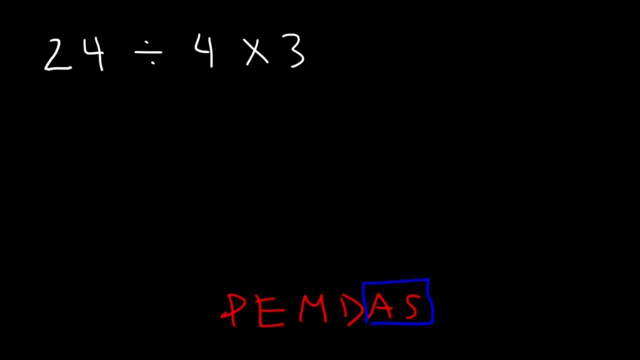 And addition and subtraction also have the same priority. Now, when you see a problem like this, where you can multiply or divide first you need to travel from left to right. That means you should work on the operations on the left and then save the operations on the right for last. 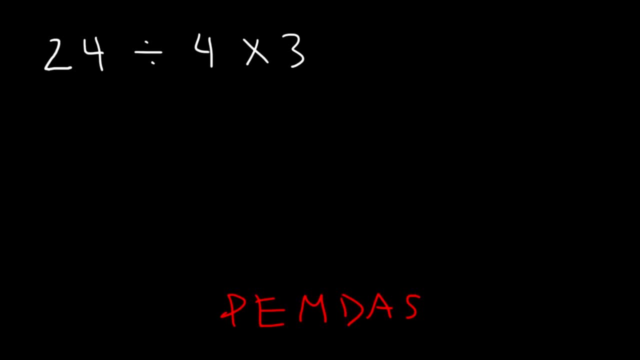 So we're going to do it two ways. Let's divide first: 24 divided by 4 is 6.. 6 times 3 is 18.. Now let's do it the other way. Let's perform multiplication first: 4 times 3 is 12.. 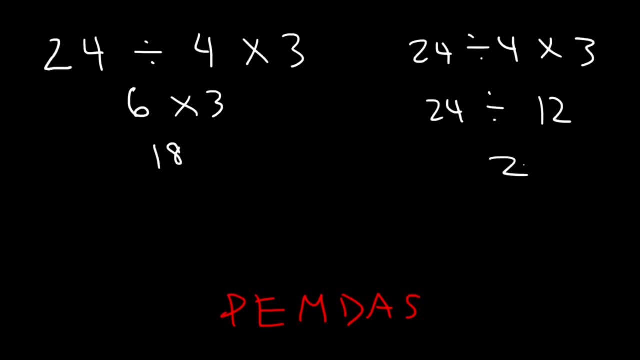 And 24 divided by 12 is 2.. So, as we can see, we get different answers here. If you type this in your calculator- hopefully you have a scientific calculator- it will give you 18 as the answer. So whenever you have division and multiplication, simply work from the left side to the right side. 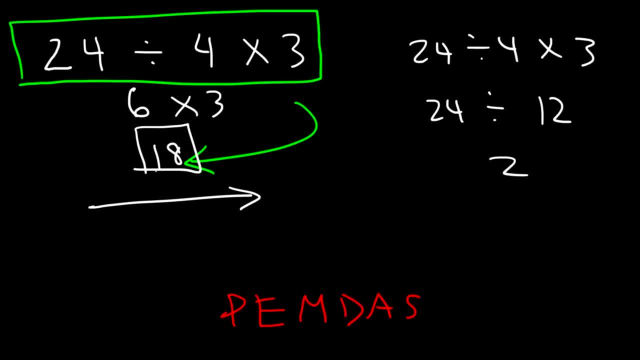 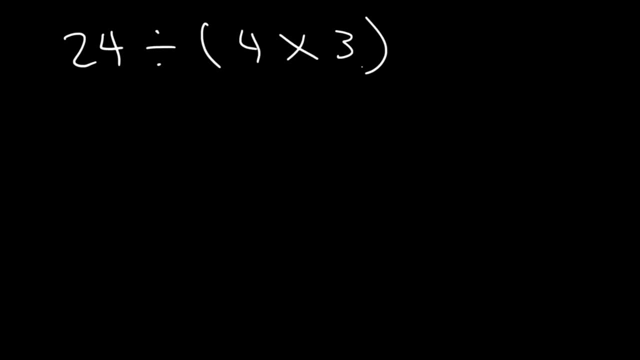 And that will give you the right answer. Now, what about a problem that looks like this In this case? what should we do? According to PEMDAS, parentheses has more priority than multiplication and division, So in this case, we need to work inside the parentheses. 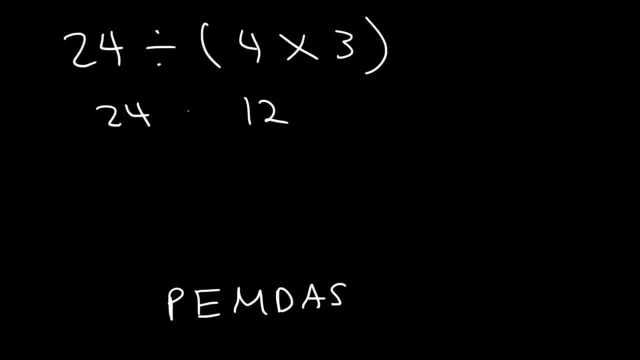 4 times 3 is 12.. And so we have 24 divided by 12,, which is 2.. And if you type this in exactly the way you see it in the scientific calculator, you should get 2 as your answer. 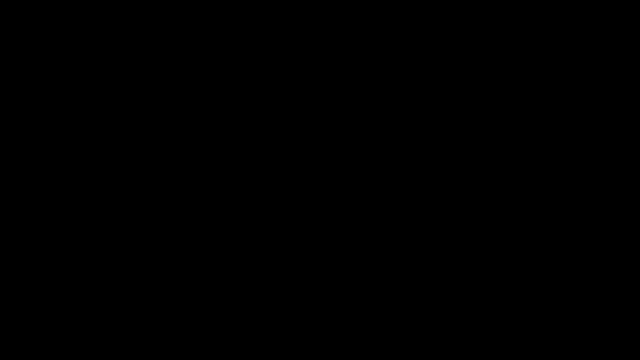 And that's how you can confirm all of these problems. Just type it in the calculator and see what you get. Now let's work on another problem. What is 48 divided by 8 minus 2? Multiply by 3.. So first we need to work inside the parentheses. 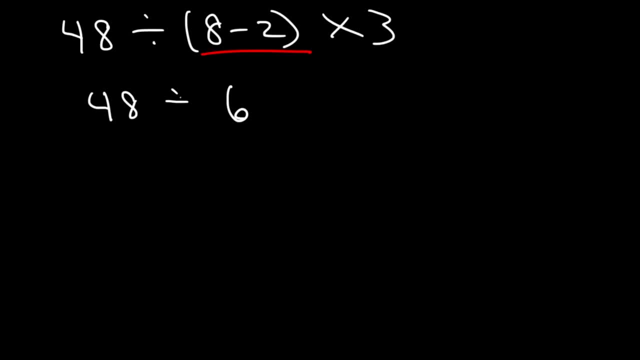 8 minus 2 is 6.. So we have 48 divided by 6 times 3.. Now that we have division and multiplication, we need to work starting from the left towards the right. 48 divided by 6 is 8.. 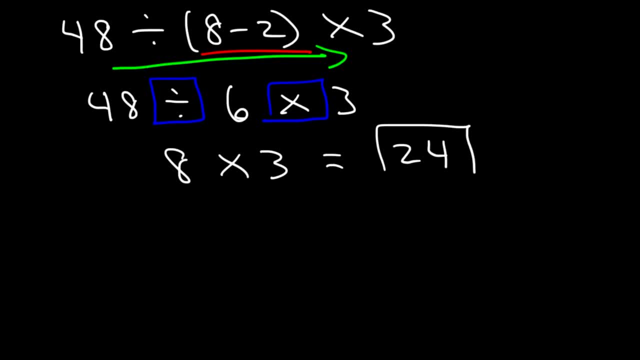 And 8 times 3 is 24.. And so that's going to be the final answer for this problem. Here's another example: What is 32 minus 24, divided by 8, divided by 2?? So feel free to pause the video and simplify this expression. 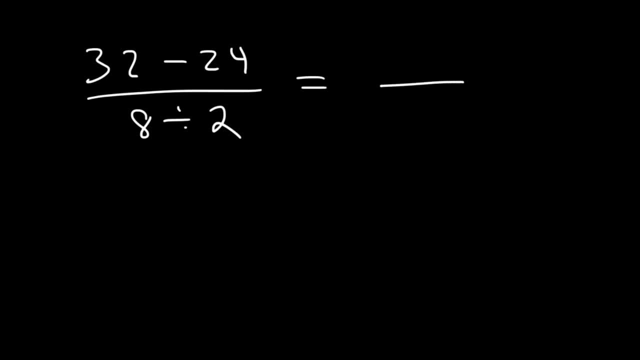 8 divided by 2 is 4.. And 32 minus 24 is 8.. And 8 divided by 4 is 2.. So that's going to be the final answer in this example. Try these two problems. What's 7 multiplied by 9 minus 4?? 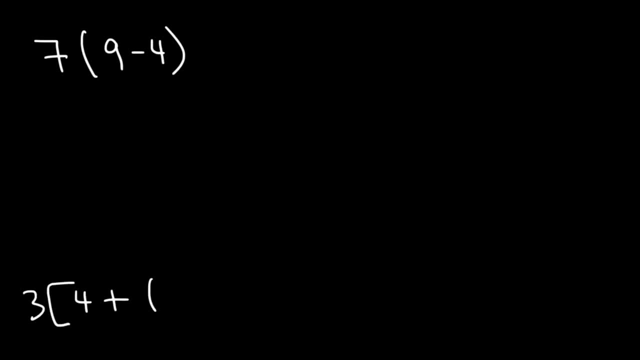 And what is 3 times 4 plus 8 minus 2 divided by 2?? So the one above is simple. We need to work inside the parentheses first. 9 minus 4 is 5.. And 7 times 5 is 35.. 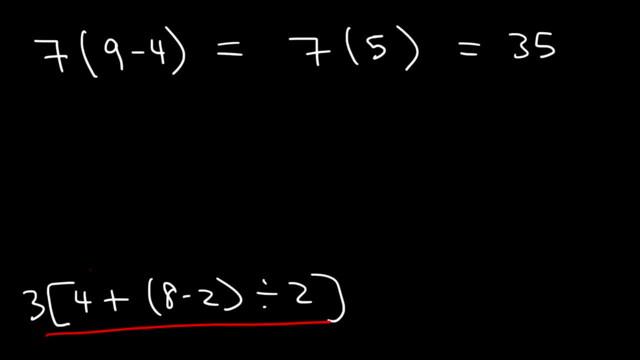 Now let's work on this example. So first we need to subtract 8 by 2.. 8 minus 2 is 6.. And now we need to work inside the brackets: 6 divided by 2, that's equal to 3.. 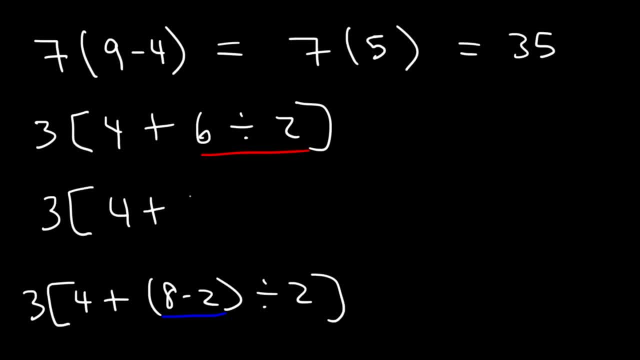 So we have 3, 4 plus 3.. Now what's our next step? 4 plus 3 is 7. And 3 times 7 is 21.. So that's the final answer for that example. Now, sometimes you may need to evaluate algebraic expressions. 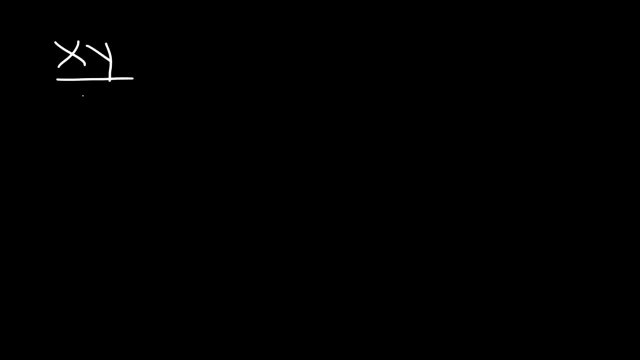 For example, let's say if we have the expression xy divided by 2 plus 5.. And let's say that you're told x is equal to 4 and y is equal to 3.. What is the value of this expression? If you see a question like this, 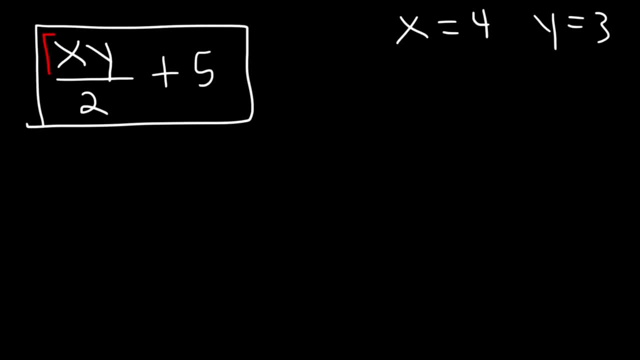 all you need to do is replace x with its value. x is equal to 4.. And y we're going to replace it with 3.. So what we now have is 4 times 3, divided by 2 plus 5.. 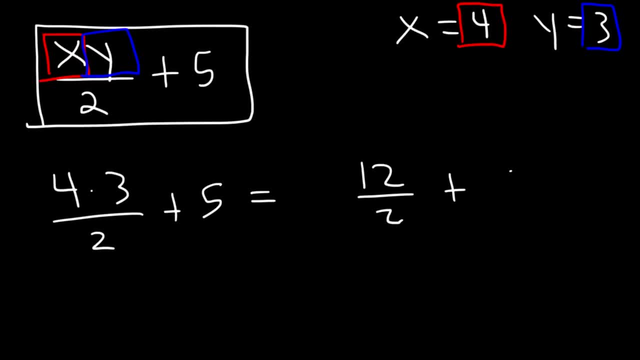 4 times 3 is 12.. And 12 divided by 2 is 6.. 6 plus 5 is 11.. So that is the value of this expression, given x equals 4 and y equals 3.. Let's work on another example. 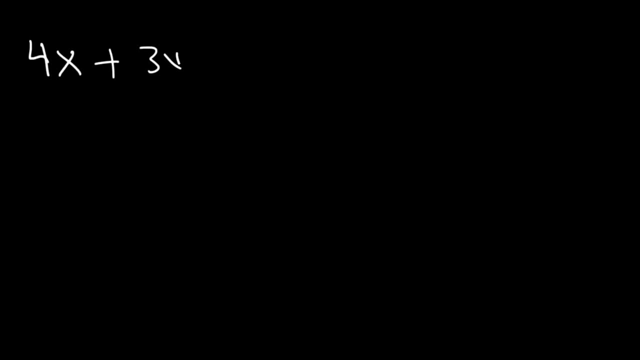 Evaluate the expression. Let's say the expression is 4x plus 3y minus 2z, And let's say that x is equal to 5, y is 2, and z is equal to 3.. So all we need to do is substitute. 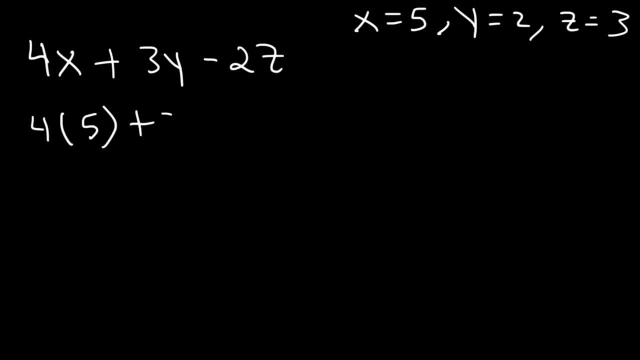 We need to replace x with its value of 5.. And we're going to replace y with 2, and z with 3.. And then just perform the operation. 4 times 5 is 20.. 3 times 2 is 6.. 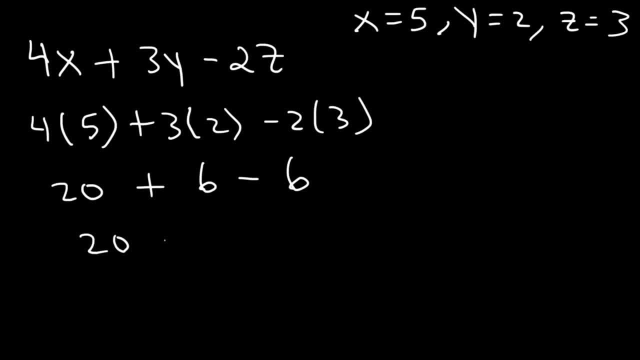 2 times 3 is also 6.. 6 minus 6 is 0. And 20 plus 0 is simply 20.. So, therefore, that's the value of this expression. Let's try another example: What is 5x minus 2 times y plus z? 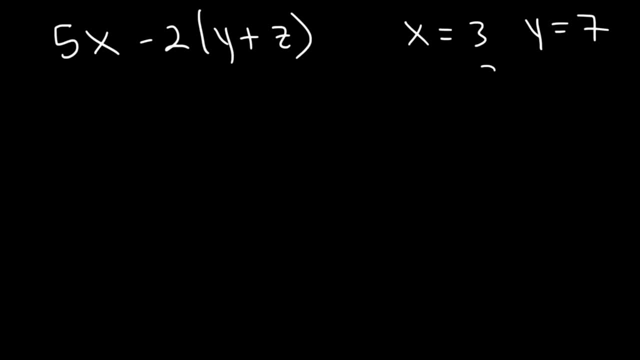 So let's say x is 3,, y is 7, and z is 4.. So feel free to pause the video and evaluate this expression. So let's replace x with 3, and y with 7, and z is 4.. 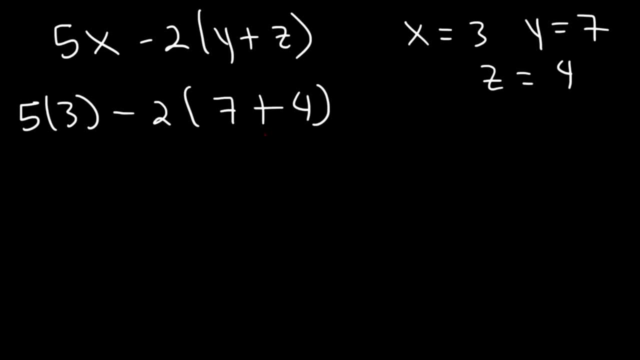 So don't forget to perform order of operations. We need to add 7 plus 4.. We could multiply 5 times 3 simultaneously. That's going to be 15.. 7 times 4 is 11.. Now we need to multiply before we subtract. 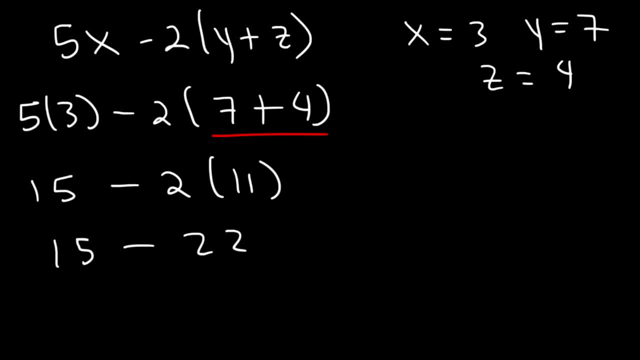 2 times 11 is 22.. So what we have is 15 minus 22,, which will give you negative 7.. And so that's the end result for this problem. Try this one: x squared minus y squared, divided by 4z plus 8.. 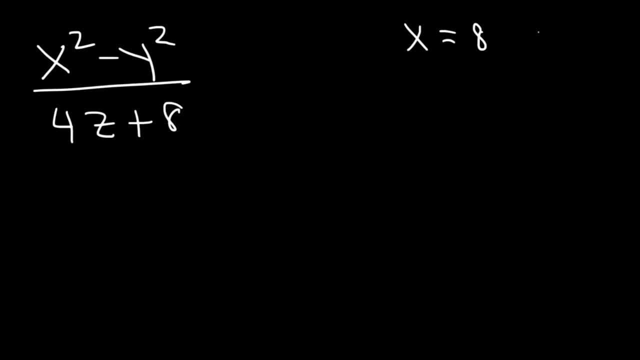 And let's say that x is equal to 8.. y is 6.. And let's say z is 4.. So x squared will be replaced with 8 squared, And y let's replace it with 6.. And then let's substitute z with 4.. 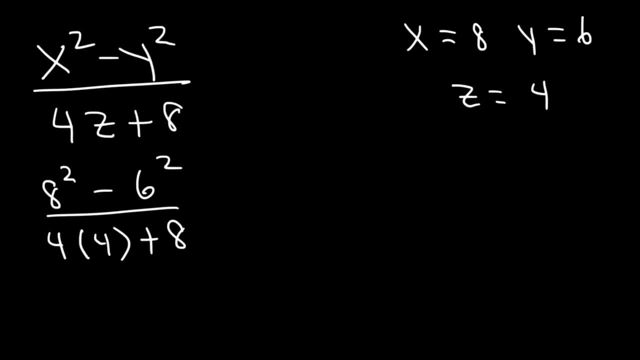 So this is the expression that we need to simplify. So now, what is 8 squared? 8 squared is 8 times 8, which is 64.. 6 squared, or 6 times 6,, that's equal to 36.. 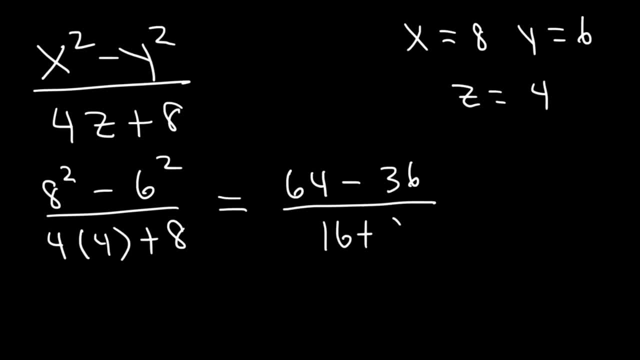 And on the bottom we have 4 times 4, which is 16.. Now what is 64 minus 36?? If we use a calculator, that's equal to 28.. And 16 plus 8 is 24.. Now this fraction is reducible. 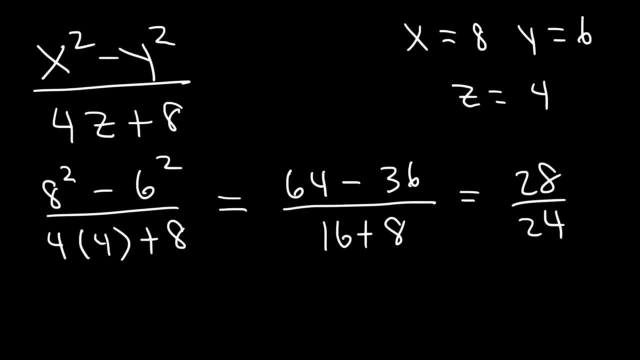 So how can we reduce this improper fraction? 28 is 7 times 4.. 24 is 6 times 4.. 4 divided by 4 is 1, so we can cancel it. So what we have left over is 7 divided by 6.. 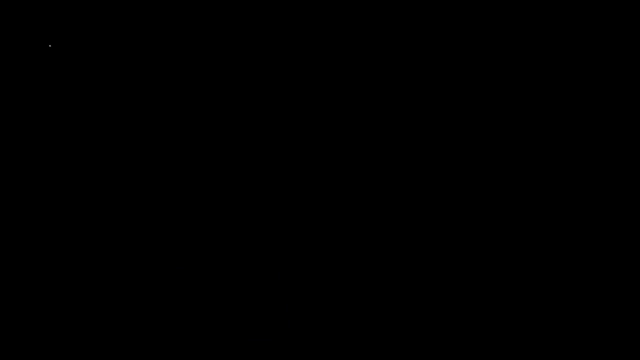 And that is the answer. What would you do if you saw an expression that looks like this: What is 3 times x plus 4?? So we can't really add x plus 4.. x is a variable in which we don't know or have a value for. 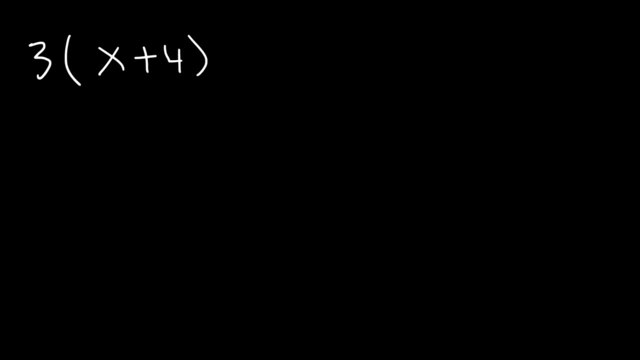 So we can't evaluate the expression, but we can simplify it. So how can we do so? Now, there's something called the distributive property. We need to distribute 3 to x and 4.. 3 multiplied by x is simply 3x. 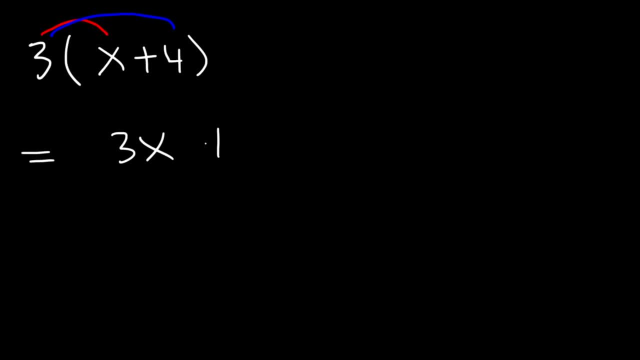 And 3 multiplied by positive 4 is 12.. So this expression is equal to 3x plus 12.. Let's try another example Now. what is 4 multiplied by 2x minus 3?? Go ahead and use the distributive property. 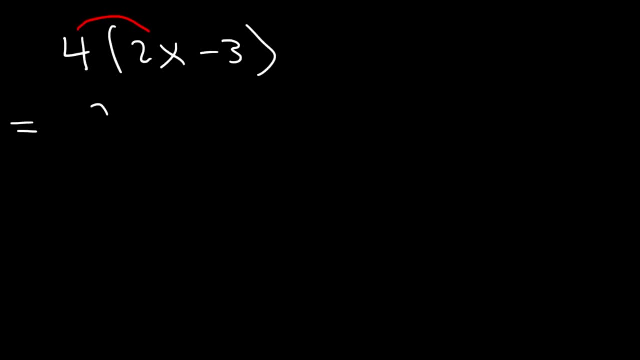 4 multiplied by 2x is equal to 8x, And 4 multiplied to negative 3 is negative 12.. So this is equal to 8x minus 12.. Now, sometimes you may have some other algebraic expressions to simplify. 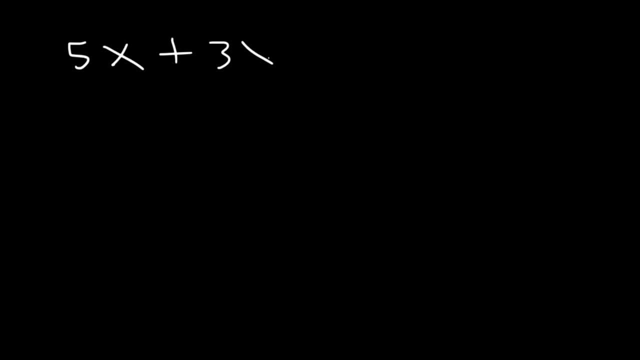 Here's another one. What is 5x plus 3x? Go ahead and simplify. All you need to do is add the coefficients. 5 plus 3 is 8.. So this is equal to 8x. Now what about this? 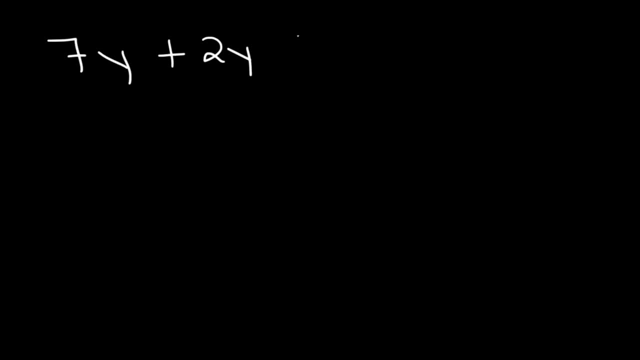 What's 7y plus 2y plus 8?? So, based on the last example, go ahead and simplify this expression. What we need to do is add, like terms: 7y plus 2y, That's equal to 9y. 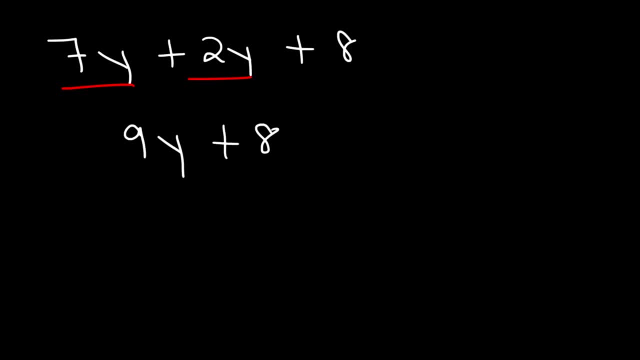 Now we cannot add 9y and 8, because what is it going to be, 17 or 17y? Because the 8 doesn't have a y. it's not a similar term to 9y, So we cannot add them. 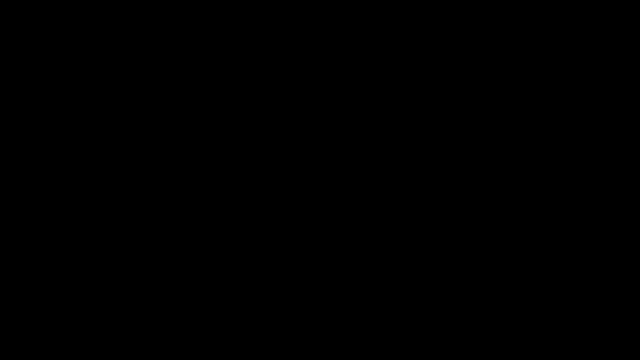 Therefore, the final answer is 9y plus 8.. Try this one 3 times x plus 5, added to 8x. Now, before we could do anything, we need to perform or use the distributive property. So we got to distribute 3 to x, which we know it's going to be 3x. 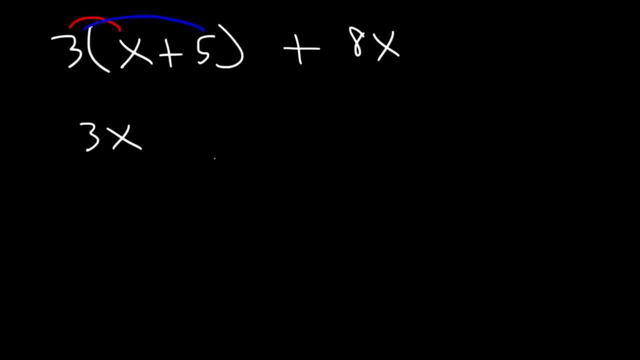 And we have to multiply 3 and 5, which is 15.. Now the only common terms that we have are 3x and 8x. They're similar. They both carry the variable x. 3 plus 8 is 11.. 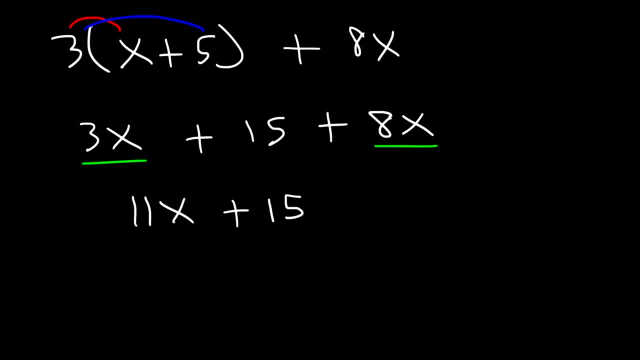 So 3x plus 8x is 11x. Therefore, the final answer is 11x plus 15.. Here's another problem that you could try: 9x plus 5 minus 3x plus 8.. Go ahead and simplify the algebraic expression. 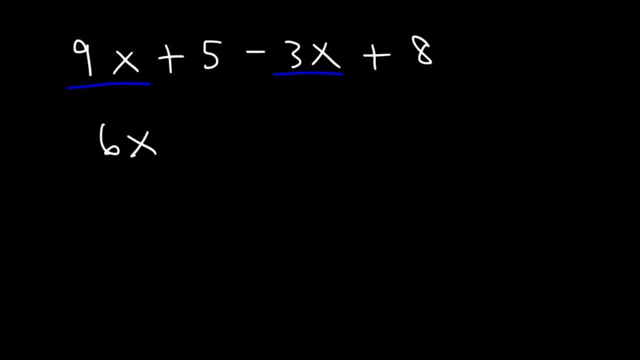 9x minus 3x is equal to 6x, And 5 plus 8, well, that's 13.. And so this is the answer: 6x plus 13.. Now let's move on to solving simple linear equations. 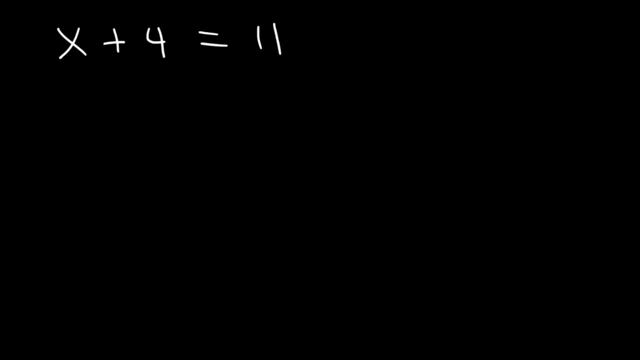 So here's an example: x plus 4.. x plus 4 is equal to 11.. What is the value of x? So, x is simply a number which you currently don't know the value of. So ask yourself what number plus 4 is equal to 11?? 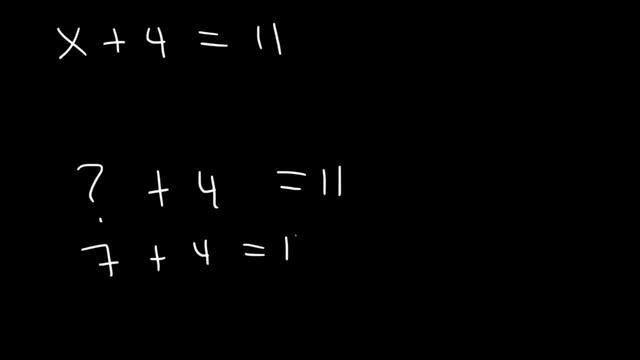 Intuitively, you know that 7 plus 4 is 11.. So therefore x has to be equal to 7.. But what can you do to show that x is equal to 7?? You understand that 7 plus 4 is 11, but mathematically how do you show that? 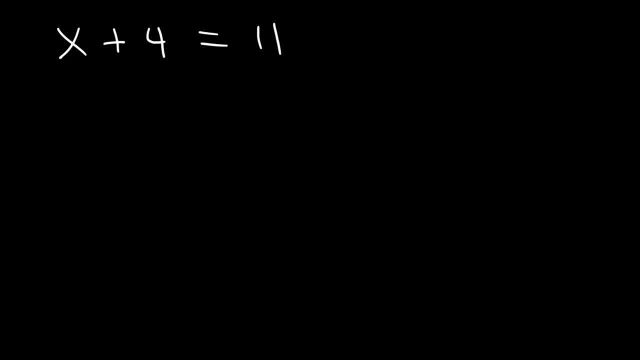 In order to find the value of x, you need to isolate x, You need to get it by itself on one side of the equation, And all other numbers you must move to the other side of the equation. So we need to get rid of this 4 on the left side. 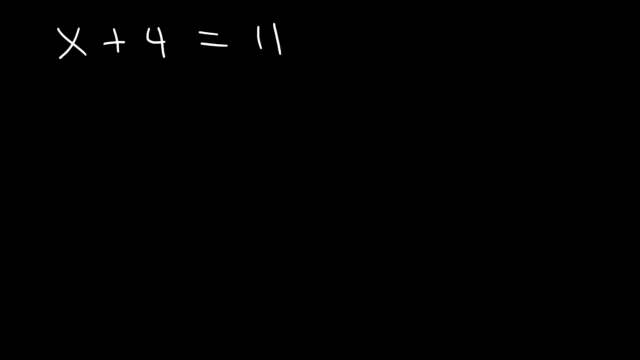 The opposite of addition is subtraction. So if we subtract both sides by 4, we can get rid of the positive 4 on the left. 4 plus negative 4 is 0. And 11 minus 4 is 7.. Any number added to 0 will be equal to that number. 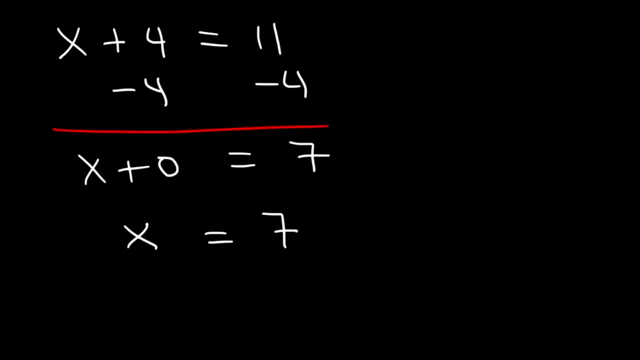 So x plus 0 is simply x. Therefore, x is equal to 7.. Here's one you should work on: y plus 5 is equal to negative 4.. What is the value of y? Well, just like before, we need to isolate y. 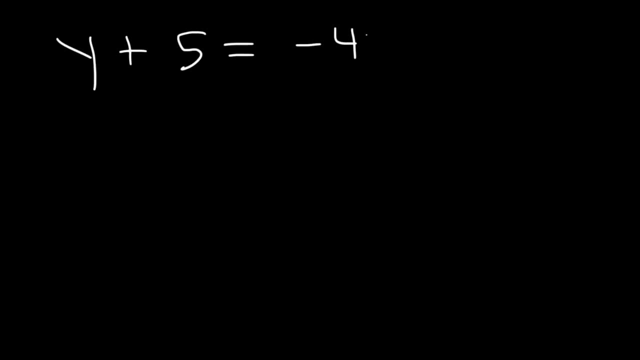 We need to get the y variable by itself, And so to remove the positive 5 on the left, we need to subtract both sides by 5.. So positive 5 and negative 5 adds up to 0, which is nothing. 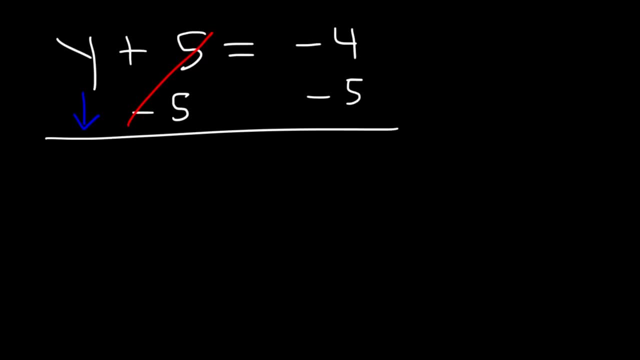 So what we have left over on the left side is simply y. On the right side, we have negative 4 plus 7.. Negative 4 plus negative 5, or simply negative 4 minus 5, which is equal to negative 9.. 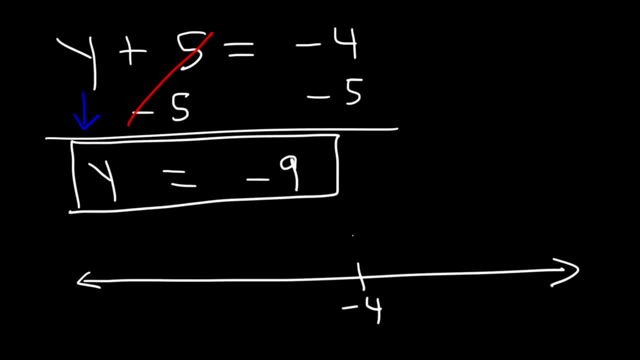 If you use the number line technique, if you start with negative 4 and travel 5 units to the left, you should get negative 9.. This is negative 5, negative 6, negative 7, negative 8, negative 9.. 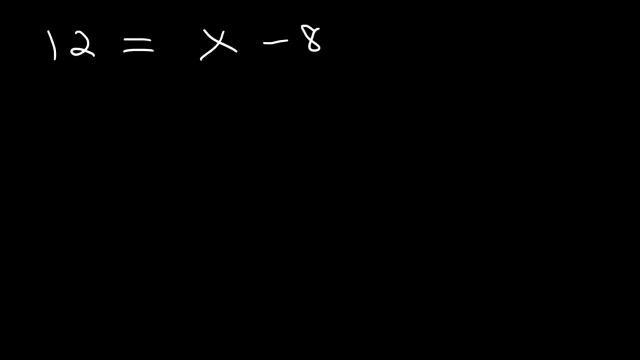 Let's say that 12 is equal to x minus 8.. What is the value of x? So x doesn't have to be on the left side, It can be on the right side by itself if we want to find the value of it. 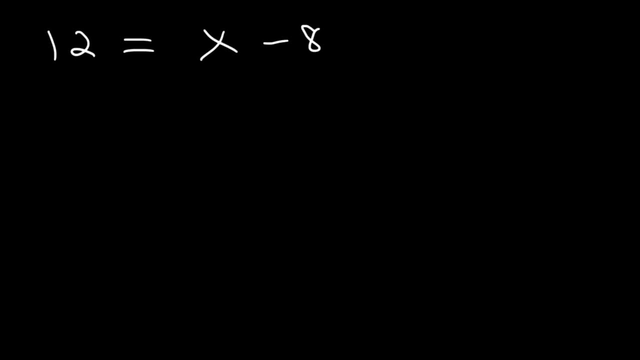 So we've got to move the negative 8.. We need to get rid of it on the right side. So the opposite of subtraction is addition. So let's add 8 to both sides. So this will cancel. We can bring down the x. 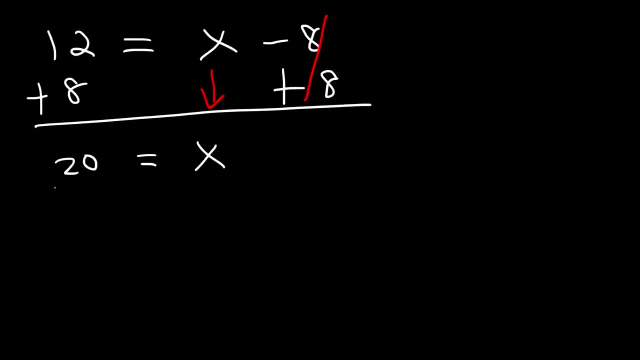 And on the left side, we have 12 plus 8, which is 20.. And so that is the value of x. Now, what about this one? 3y is equal to 18.. What is the value of y? So we need to separate 3 from y. 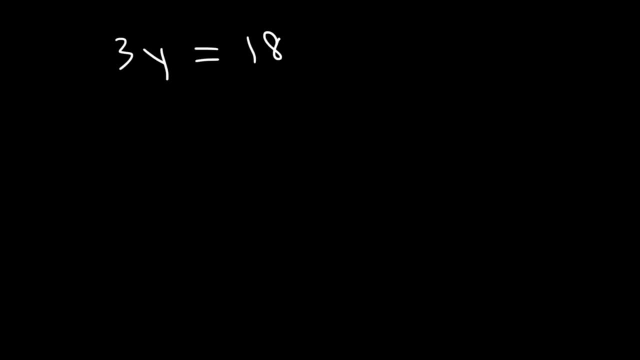 Currently, the 3 is multiplied to y. The opposite of multiplication is division, So therefore we need to divide both sides by 3.. 3 divided by 3 is 1. And 18 divided by 3 is 6.. 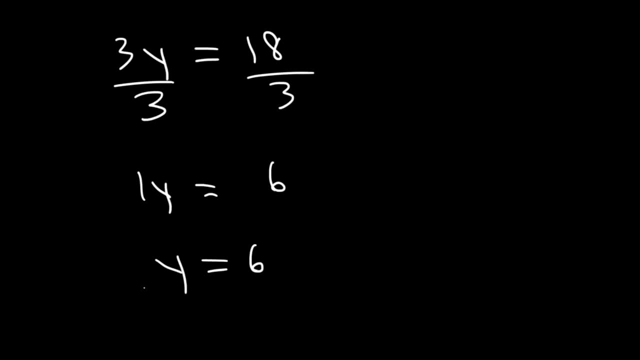 1y is the same as y, So therefore y is equal to 18.. y is equal to 6.. So if we look at this expression 3 times, what number is 18?? We know that 3 times 6 is 18.. 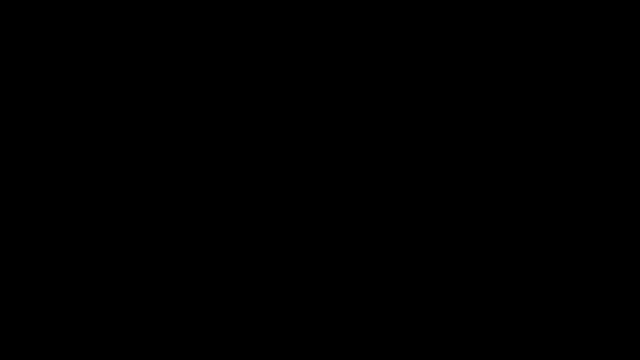 So therefore, y is equivalent to 6.. Now what if you saw an example like this: 8 is equal to x divided by 4.. What should you do to find the value of x? So x is divided by 4.. And the opposite of division is multiplication. 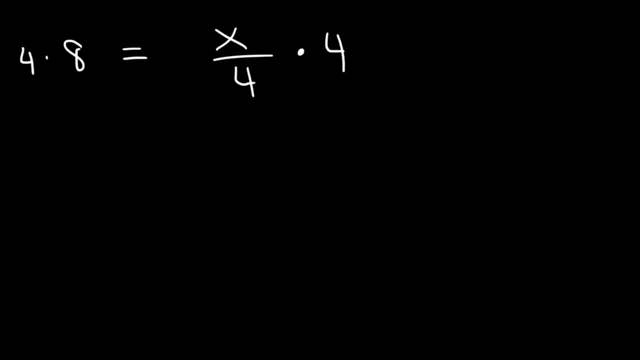 Therefore, we need to multiply both sides by 4.. And that's how we can get rid of the 4 on the right side. 4 divided by 4 is 1.. And so we just have x on the right side. On the left, we have 4 times 8, which is 32.. 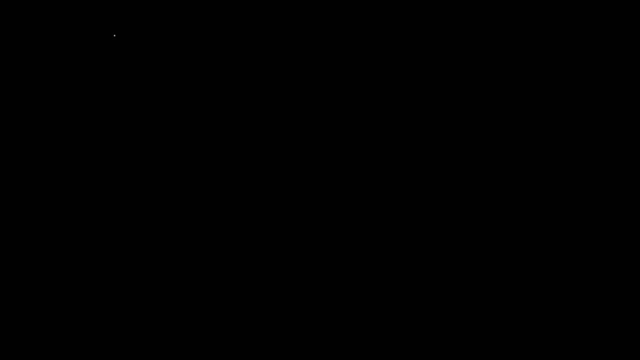 So x is 32.. Now, what about this one? Now, what about that one? 2 thirds x is equal to 9.. How can we find the value of x If you have a fraction in front of the variable that you want to isolate? 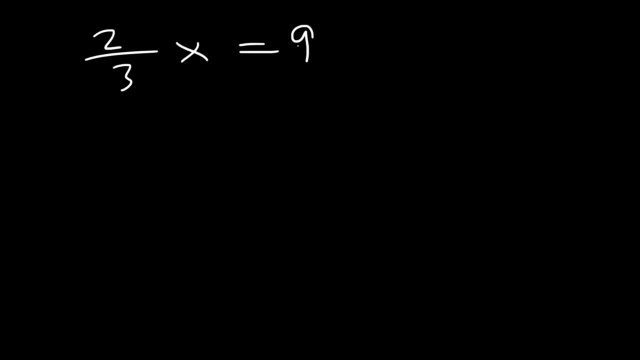 multiply both sides by the reciprocal of the fraction, So that is, multiply both sides by 3 over 2.. 9 is the same as 9 over 1.. Now, whatever you do to the left side, you must always do to the right side. 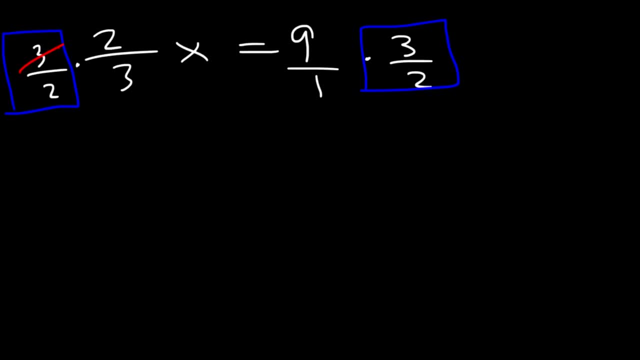 3 divided by 3 is 1. And 2 divided by 2 is 1.. So the 2's and 3's cancel on the left. On the right, we have 9 times 3, which is 27.. 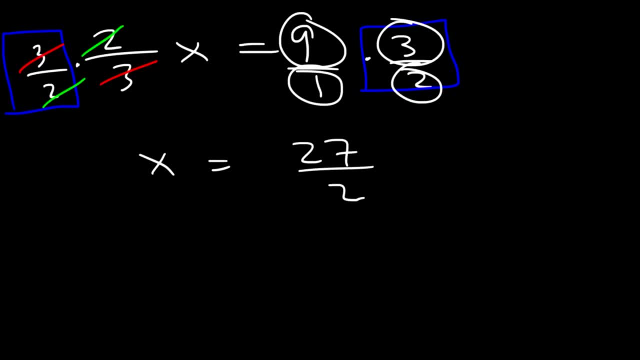 And 1 times 2, which is 2.. So the answer is 27 divided by 2.. Now we could simplify this fraction if we want to. 27 is 26 plus 1. And 26 divided by 2 is 13.. 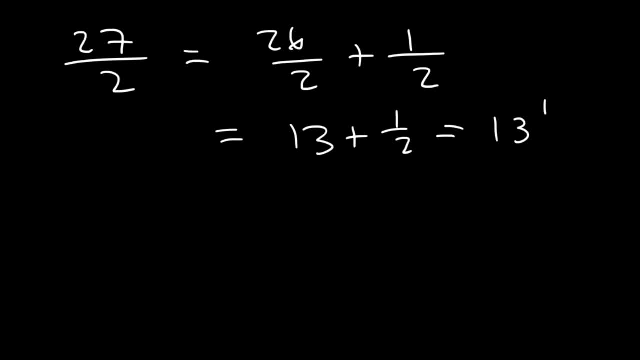 13 plus 1 half is 13 and 1 half as a mixed number. So as a decimal this is equal to 13.5.. So that is the value of x in this problem. Try this: one x plus 3 divided by 4 is equal to 10 over 5.. 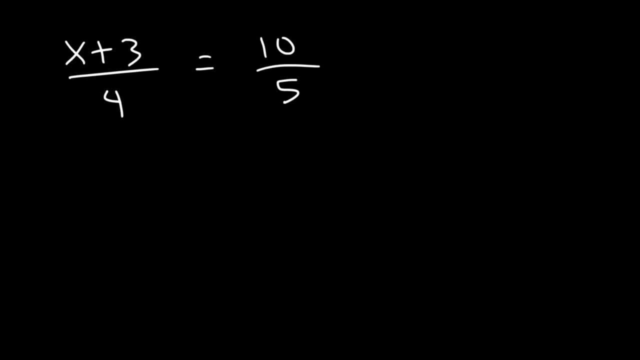 Now, what can we do to find the value of x? What can we do to find the value of x if we have two fractions separated by an equal sign? If you see this, the best thing you could do is cross, multiply 4 times 10 is 40.. 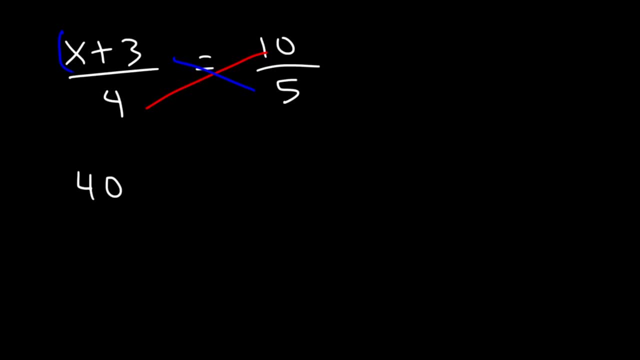 And 5 times x plus 3, we need to distribute the 5.. So 5 times x is 5x, And 5 times 3 is 15.. So this is what we now have. Our next step is to subtract both sides by 15.. 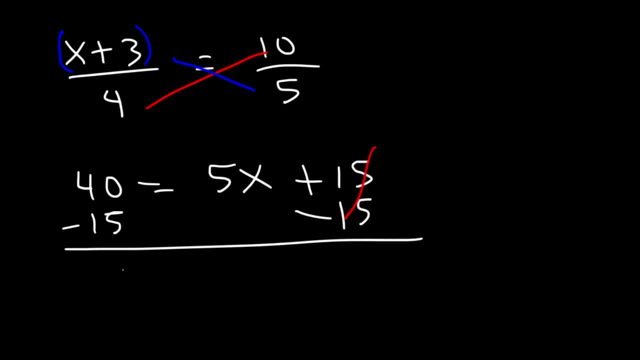 40 minus 15 is 25.. So 25 is equal to 5x. Next, we need to divide both sides by 5.. 25 divided by 5 is 5.. So x is equal to that number. Go ahead and try this. 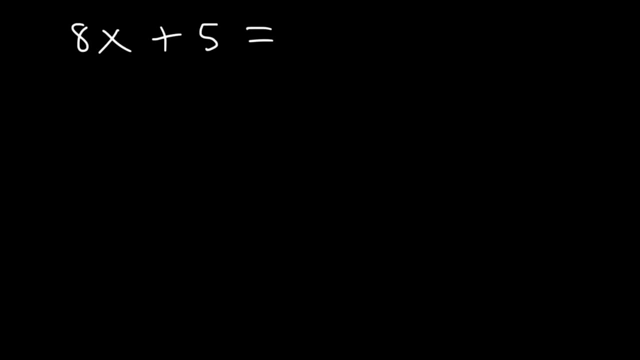 In that last example we solved an equation that looks like this after cross multiplying. So this is a multi-step equation. Now, before separating 8 and x, you need to get rid of the 5 on the left side. So the opposite of addition is subtraction. 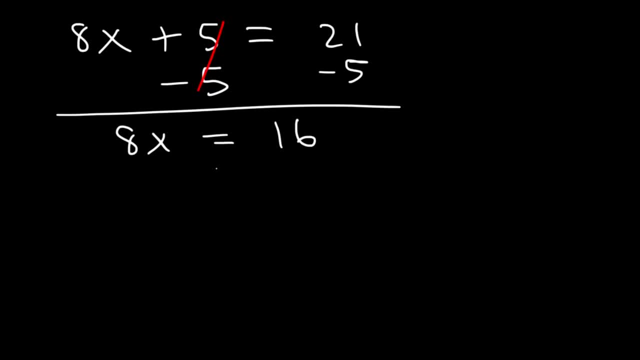 21 minus 5 is equal to 16.. And now we need to divide both sides by 8 to separate x from 8.. So 16 divided by 8 is 2. And that is the value of x in this example. 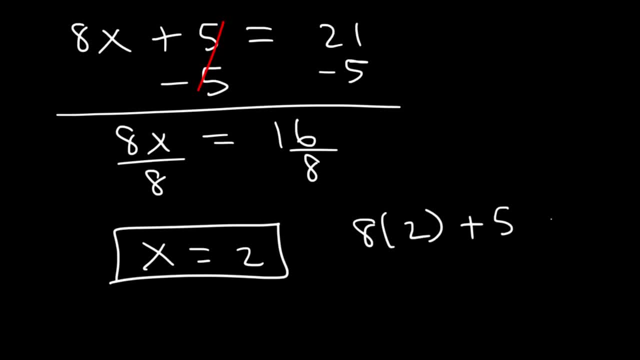 And we can check it: 8 times 2 plus 5. Is that equal to 21?? 8 times 2 is 16.. 16 plus 5 is 21.. So x is indeed equal to 2.. Go ahead and try this one. 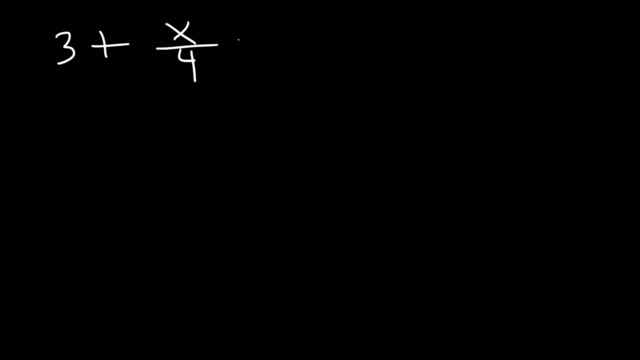 Let's say that we have 3 plus x divided by 4.. And let's say that's equal to 5.. What is the value of x? There's many ways in which you could solve it, But if you want to get rid of the fraction, multiply everything by 4.. 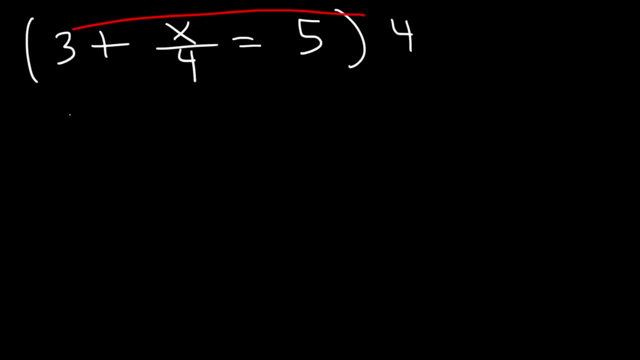 So 4 times 3 is 12.. x divided by 4 times 4.. The 4's will cancel, leaving behind x. And then we have 4 times 5,, which is 20.. And now all we need to do is subtract both sides by 12.. 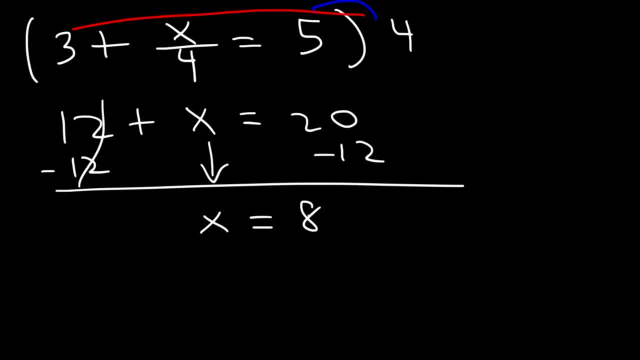 20 minus 12 is 8. And so that is the value of x. So if you're solving a linear equation and if you have fractions, it's helpful to multiply every term by the denominator of the fraction, just to clear away all fractions. 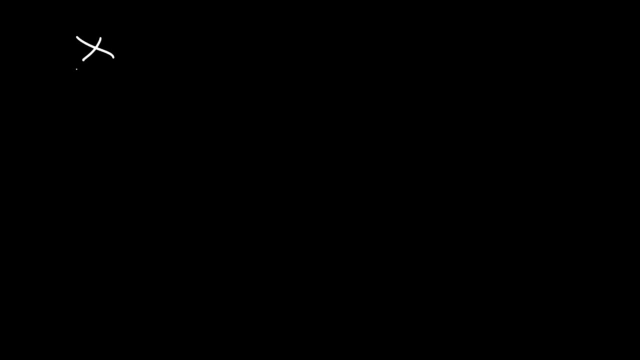 Now what about this one? Sometimes you may have multiple fractions. What is the value of x In this case? multiply by a multiple of 2,, 3, and 4.. 12 is the least common multiple of 2,, 3, and 4.. 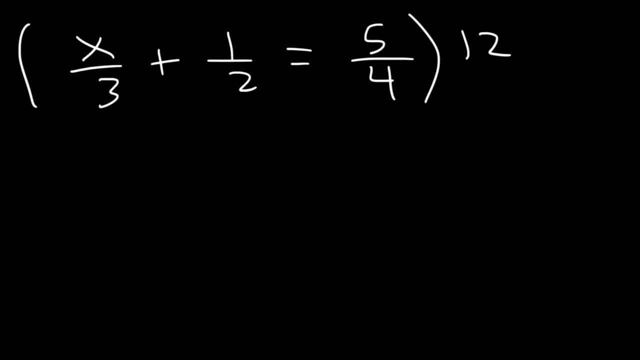 12 is divisible by 2, 3, and 4.. So first let's multiply 12 by x divided by 3.. So that's going to be 12x divided by 3, which is 4x. And then let's multiply 12 by 1 half. 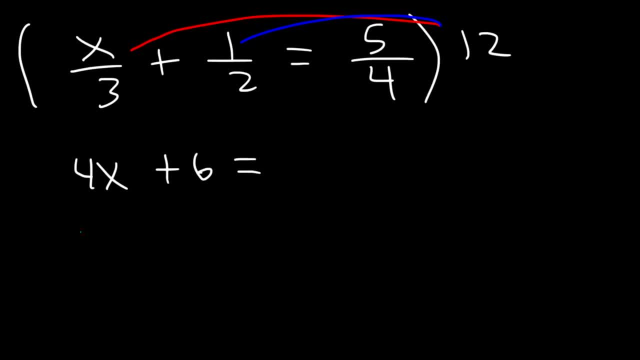 Half of 12 is 6.. Now what is 12 times 5 fourths? There's two ways in which you can do this. You can multiply first and then divide, or divide first and then multiply. 12 times 5 is 60.. 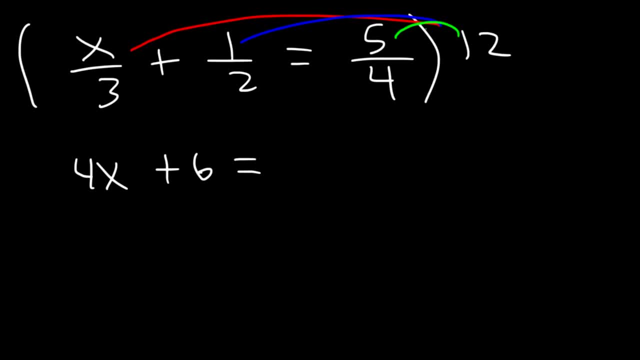 60 divided by 4 is 15.. Or you could say: 12 divided by 4 is 3.. 3 times 5 is 15.. So either case, you're going to get the same value. Now let's subtract both sides by 6.. 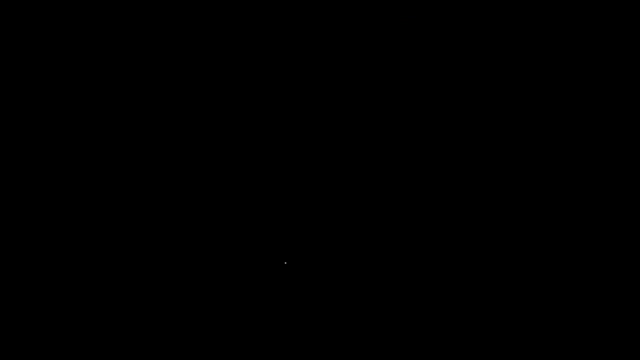 15 minus 6 is 9.. So we have: 4x is equal to 9.. Let's divide by 4.. So now we have an improper fraction. x is 9 over 4. And that is the answer. If you want to convert it to a mixed number. 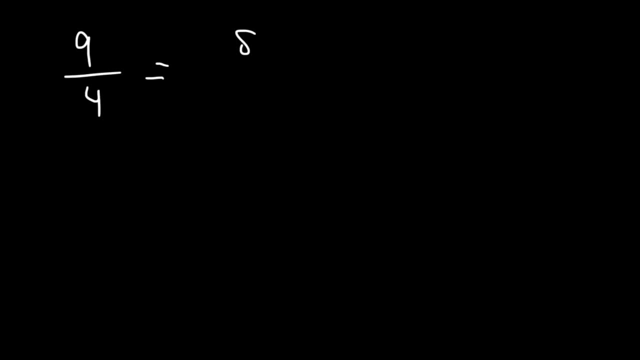 separate 9 into 8 and 1.. 8 plus 1 is 9.. 8 divided by 4 is 2.. So we have 2 plus 1 fourth, Which is the same as 2 and 1 fourth as a mixed number. 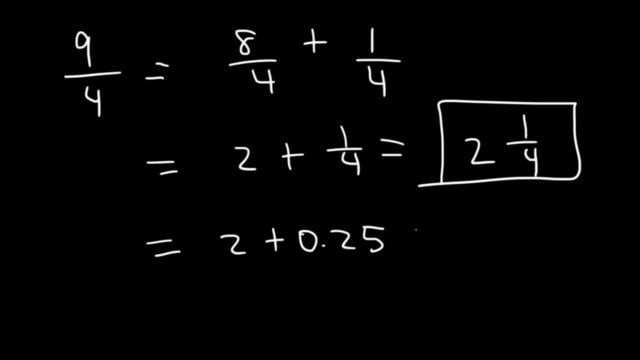 As a decimal. 1. fourth is .25.. So 9 over 4 is equivalent to 2.25.. Now let's spend a moment talking about exponents. So what is 2 raised to the third power? What is that equal to? 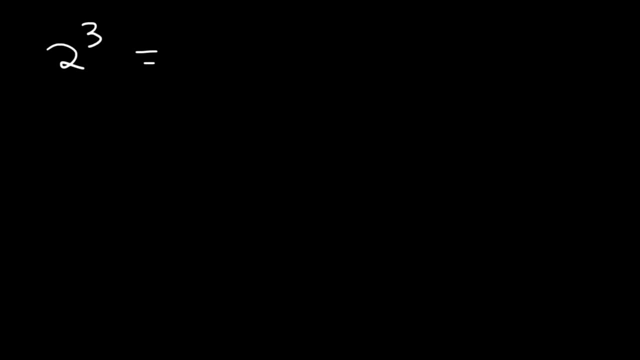 Having exponents suggests repeated multiplication And, if you recall, multiplication is repeated addition. So 2 to the third power means that you're multiplying 3, 2's together, Which is equal to 8.. 4 to the third means that you're multiplying 4 times, 4 times 4.. 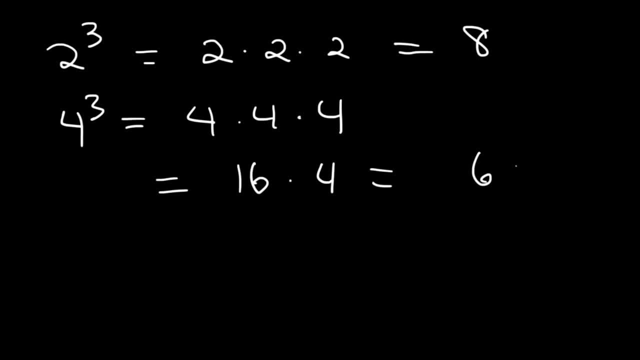 4 times 4 is 16.. 16 times 4 is 64. So 4 to the third is 64.. Now what is the value of these three expressions: Negative 2, squared. Negative 3, squared. And negative 3- inside a parenthesis: squared. 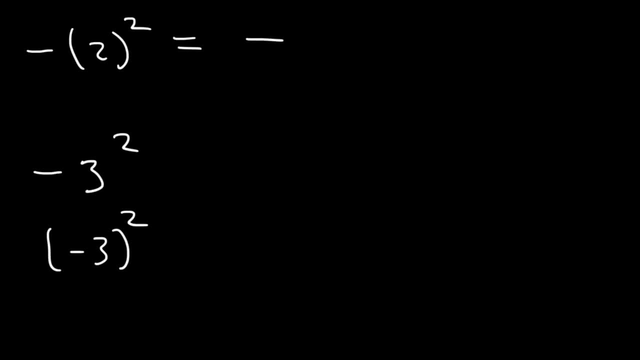 So above we have a negative And we're multiplying 2- 2's. The 2 is positive and we have 2 of them. So 2 times 2 is 4.. Combined with a negative sign, that's negative 4.. 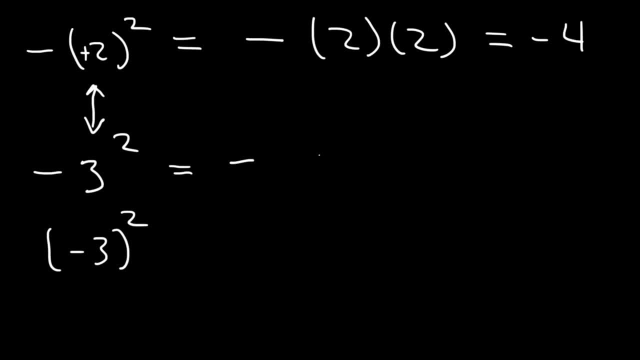 These two expressions are equivalent, So this is negative times 3 times another 3.. Which is negative 9.. On the bottom, we have two negative 3's multiplied to each other. Since the negative is inside the parenthesis, it's affected by the exponent. 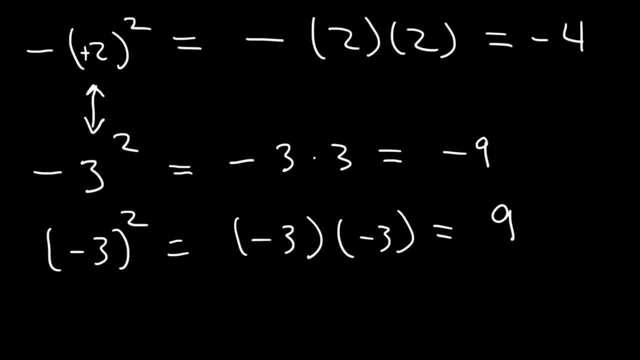 Negative 3 times negative, 3 is positive 9.. So make sure you know the difference between those expressions. Now the next thing we need to talk about is factoring binomials. For example, let's say, if we have the expression 14x. 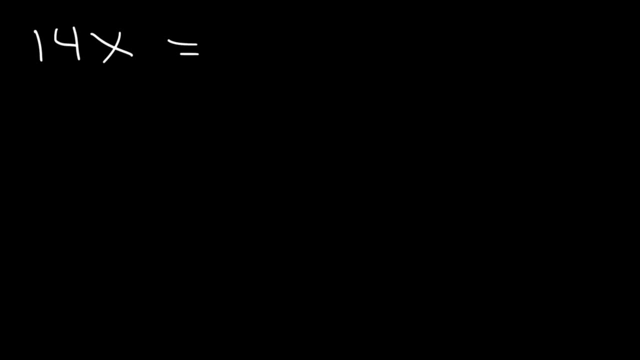 How can we factor this binomial? that is right in everything in terms of prime numbers: 14,. we can break it down into 7 times 2.. And we only have one x variable, so that's 14x. That's how you can factor it. 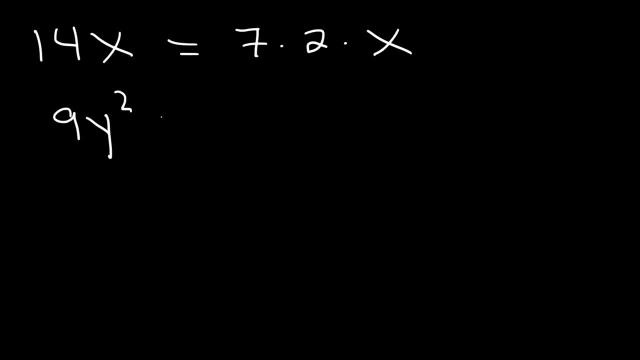 Now let's say, if we want to factor 9y squared, 9 is 3 times 3.. y squared is y times y. So that's how you can factor that binomial. Now what about 8xy squared? Go ahead and factor it completely. 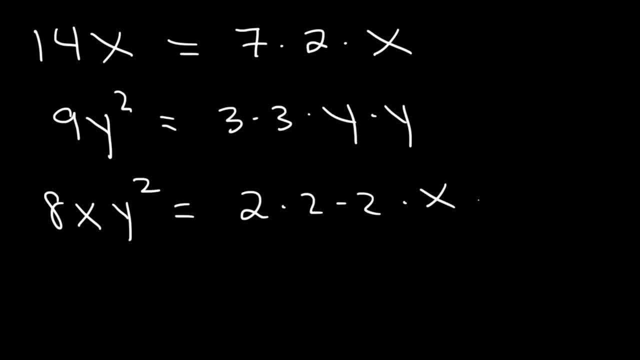 8 is basically 2 times 2 times 2.. We have one x variable and two y variables, So that's 8xy squared, Completely factored. Try these two: 28a squared, b Negative, 12x cubed y. 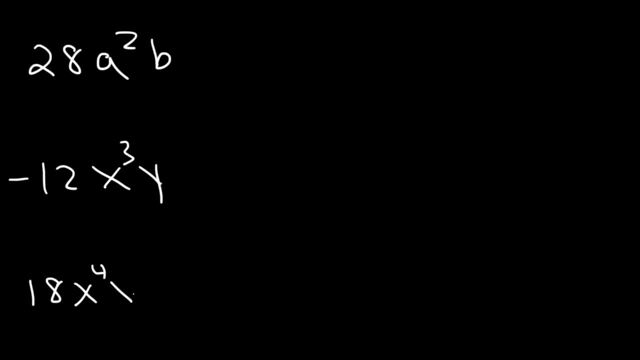 And 18x to the fourth, y to the fifth. So go ahead and factor those binomials completely. Let's start with 28.. 28 is 7 times 4.. And 4, we can break that down into 2 times 2.. 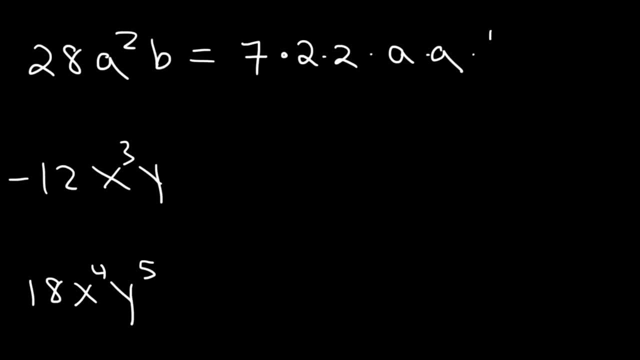 So that's 28.. a squared is a times a, And then we have one b variable: 12 is negative 4 times 3.. And 4 is 2 times 2.. x cubed is x times x times x. 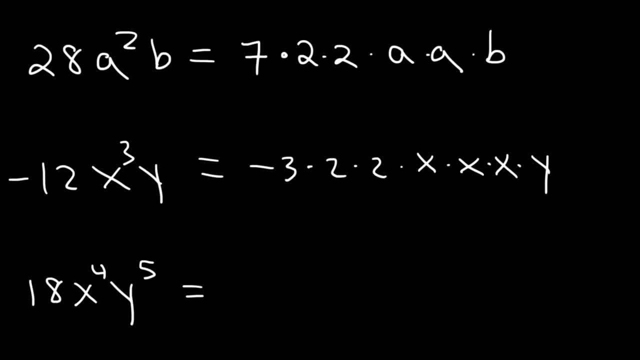 And we have a y variable. Now, 18 is 3 times 6. And 6,? we can break that down into 3 times 2.. y to the fourth means that we're multiplying 4 x variables, And y to the fifth means that we're multiplying 5 y variables together. 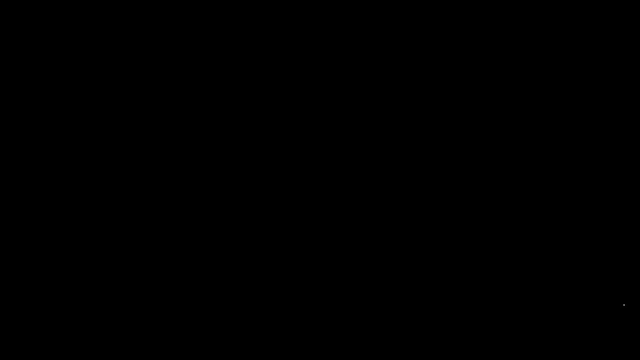 And so that is the answer. So now you know how to factor binomials completely. Now the next topic of discussion is finding the GCF, The greatest common factor. What is the greatest common factor between 8 and 12?? So look for a number that's less than 8 and 12.. 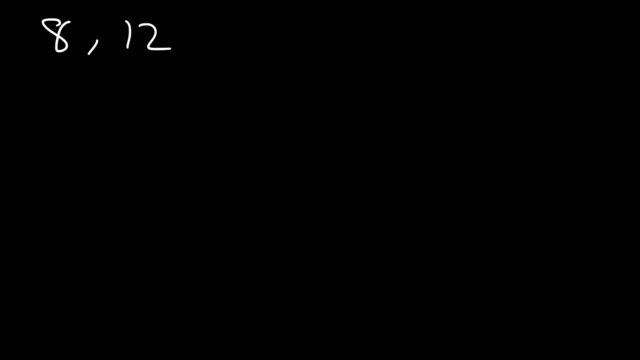 And that goes into 8 and 12.. So this number- 8 and 12, are both divisible by this integer. So what is the highest number that is divisible by 8 and 12?? So first let's factor 8 completely. 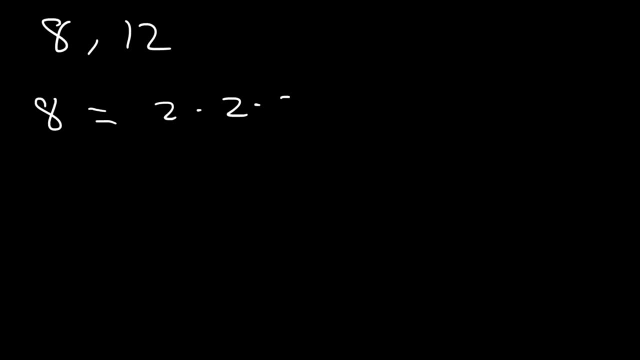 8 is 2 times 2 times 2.. 12 is 2 times 2 times 3.. So notice that 8 and 12 have these numbers in common. That is 2 times 2.. So basically it's 4.. 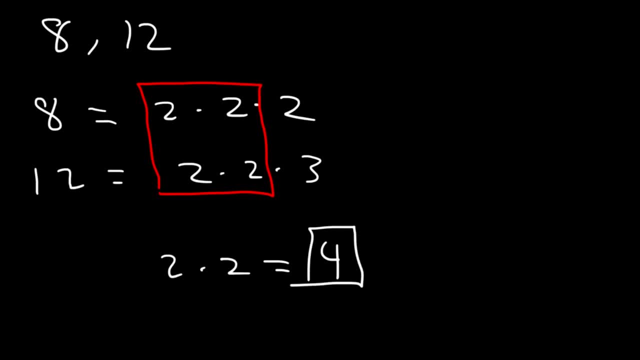 That is the greatest common factor between 8 and 12.. 8 is divisible by 4. And 12 is also divisible by 4.. Let's try another example: What is the greatest common factor between 12 and 18?? So feel free to pause the video and try that example. 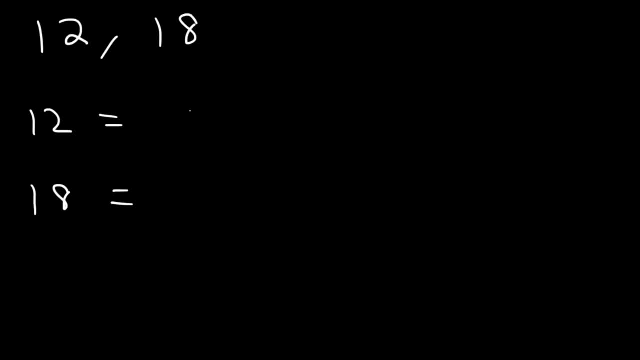 So let's find out the prime factorization of 12 and 18.. 12 is 3 times 4. And 4 is 2 times 2.. 18 is 3 times 6. And 6 is 3 times 2.. 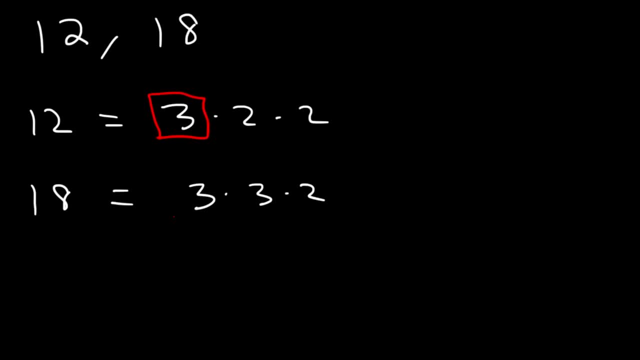 So 12 and 18 have a 3 in common And they also have a 2 in common. 3 times 2 is 6.. So that is the GCF between 12 and 18.. The greatest common factor is 6.. 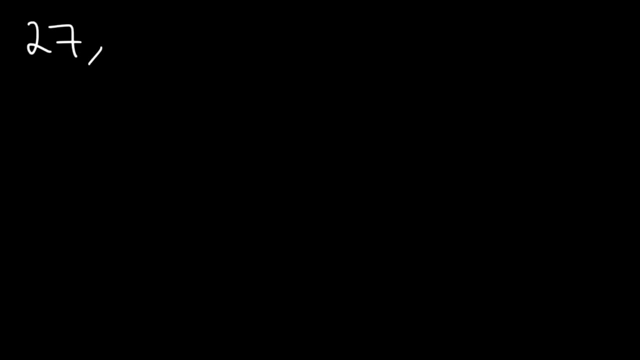 Now what is the greatest common factor between 3 numbers: 27,, 36, and 45. So go ahead and try that. 27 is 9 times 3. And 9 is 3 times 3.. So 27 is 3 to the third power. 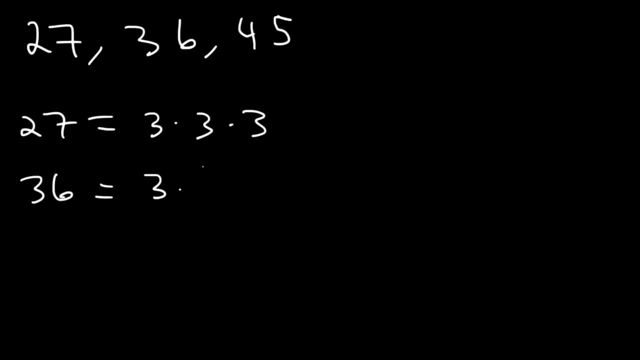 36 is 3 times 12.. And 12 is 3 times 4.. And 4 is 2 times 2.. 45 is 5 times 9. And 9 is 3 times 3.. So all of these numbers have these two in common. 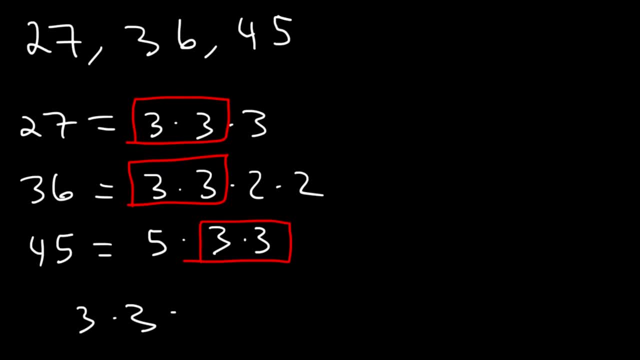 That is 3 times 3.. So the GCF between 27,, 36, and 45 is 9.. Each of those numbers are divisible By 9.. Now what about this example? What is the greatest common factor between 5xy and 10x squared y? 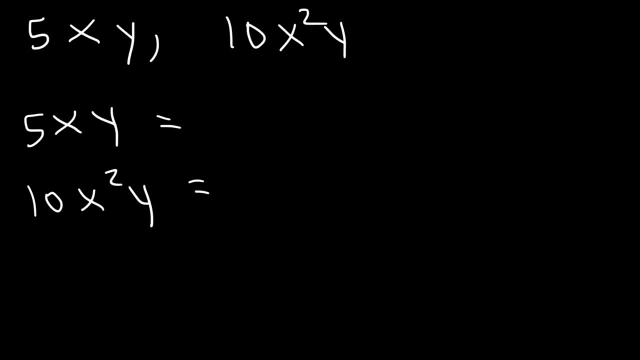 So let's follow the same process. 5xy is simply 5 times x times y. 10x, squared is 5 times 2 times x times x times y. So we have a 5 in common And we have an x in common. 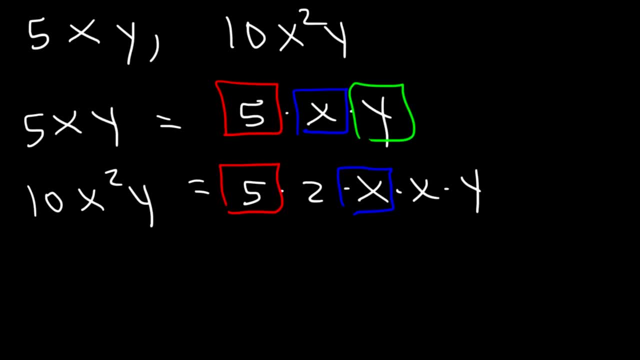 And we also have a y in common. So therefore, the greatest common factor is 5xy. Let's try this one: 6x and 9x squared y, What's the GCF? So we can factor 6x into 3 times, 2 times x. 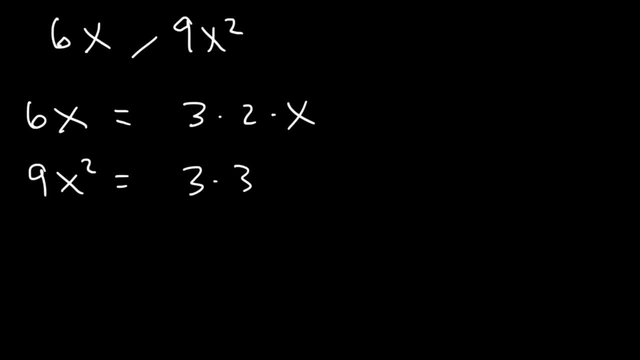 9x squared is 3 times 3 times x times x, So these two terms have 3x in common. So that's going to be the GCF. Between 6x and 9x squared, It's 3x. 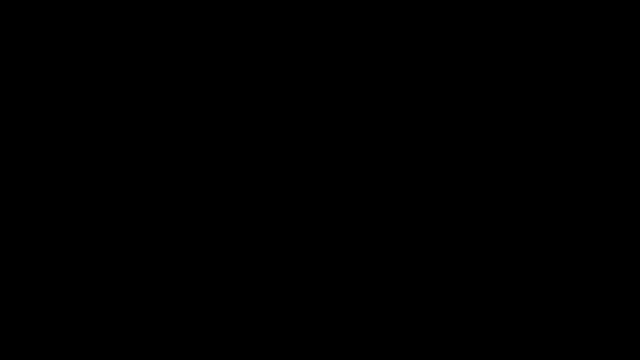 Now let's spend a few moments simplifying fractions. For example, What is 14x squared y divided by 63xy? When dividing monomials, what you can do is you can simplify it by factoring: 14 is 7 times 2.. 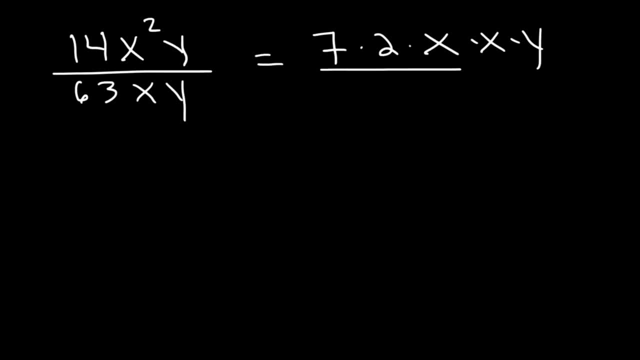 X squared is x times x, And then we have a y: 63 is 7 times 9.. And we still have an x and a y. Notice what we can cancel at this point. We can cancel a 7. And we can cancel an x and a y. 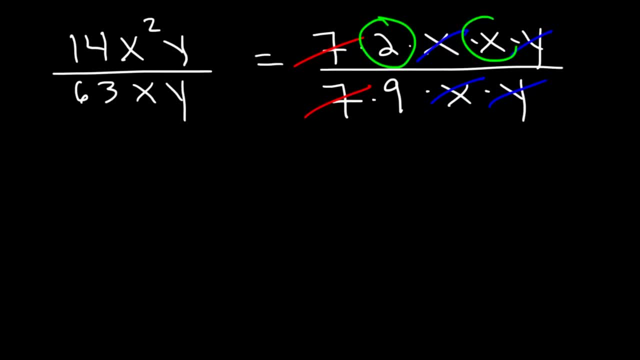 So on top, what we have left over is 2 times x. On the bottom, simply a 9.. So the answer is 2x divided by 9.. And that's how you can simplify monomials: by factoring. Let's try another example. 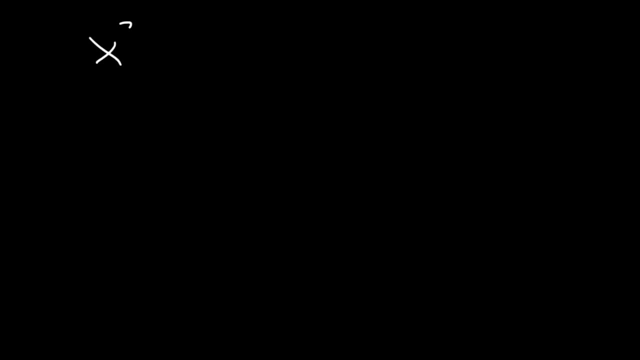 What is x squared divided by x to the 5th power? So let's simplify by factoring: X squared is x times x. X to the 5th is basically 5x variables multiplied to each other, So we can cancel 2 of them. 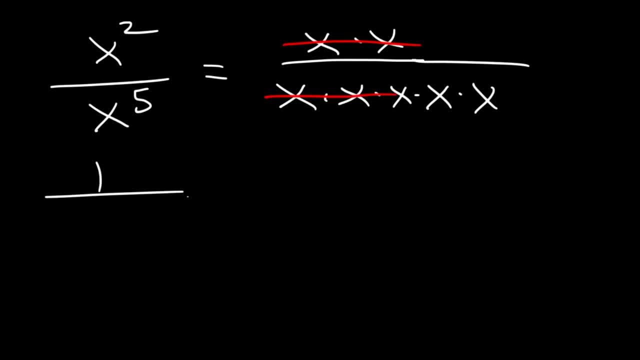 And that leaves behind 3x variables on the bottom, And x to the 5th is the same as x to the 5th times x times x is simply x cubed. so the answer is 1 divided by x cubed. Now what? 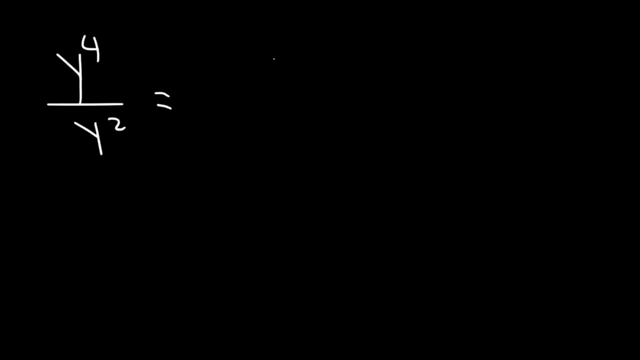 about this one: y to the fourth divided by y squared. y to the fourth is y times y times y times another one, and y squared is simply y times y. so we can cancel two of these, leaving behind y times y, which is y squared. Try this one: 21 x, y. 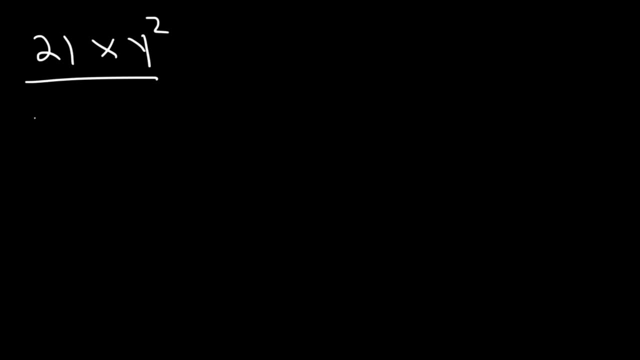 squared divided by 28 x squared y cubed. so feel free to take a moment to simplify that expression: 21 is 7 times 3 and y squared is y times y. 28 is 7 times 4 times x squared and y cubed is y times y times y. So first we 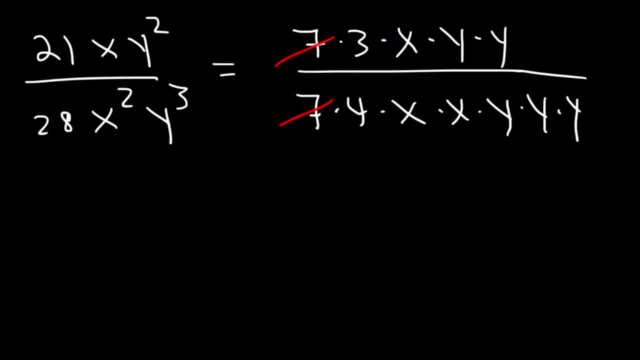 can cancel a 7 and we can cancel an x variable and we can cancel two y variables. So on top, all we have left over is a 3, and on the bottom we have a 4 and x and one y variable. so it's going to be 4- x- y. 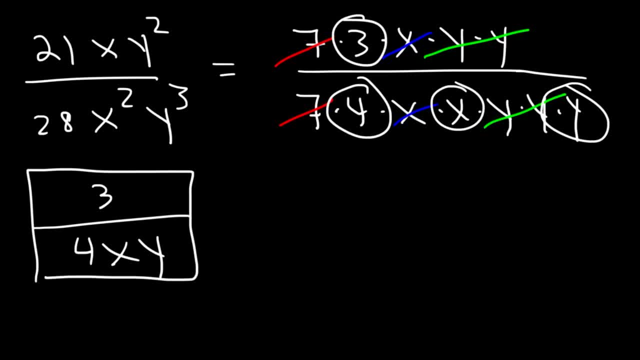 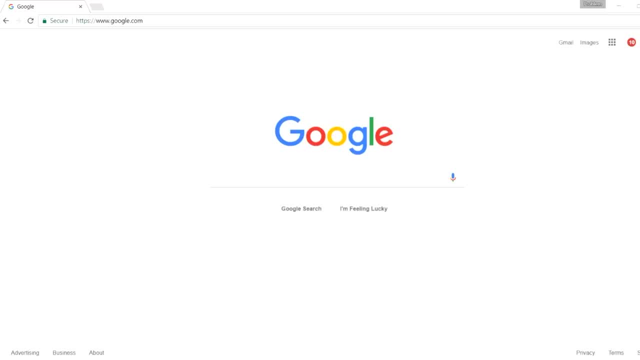 And that's the answer. So now you know how to simplify monomials when they're divided against each other. Now I'm going to show you an online algebra course that you can use to help you with other topics. So, if you go to udemycom- 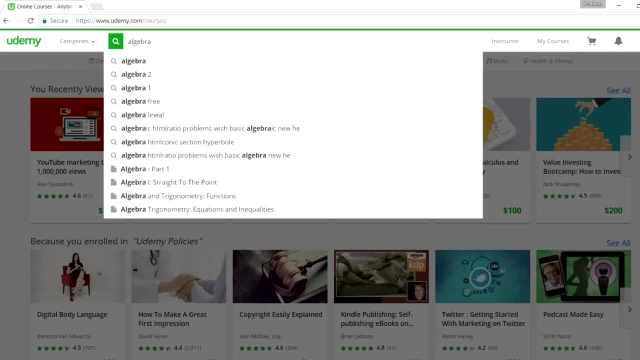 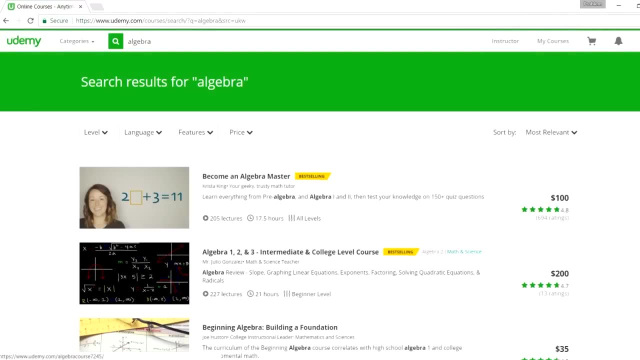 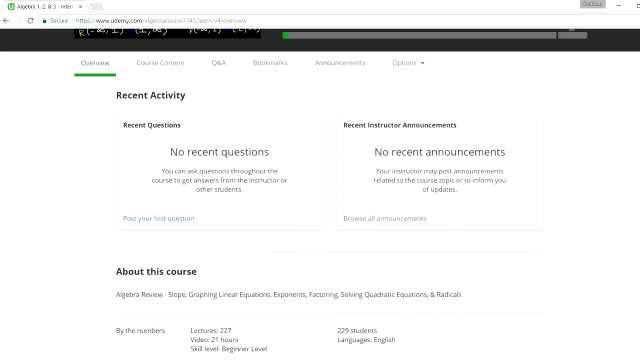 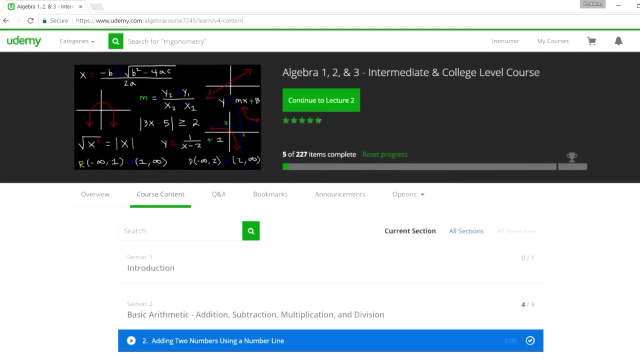 and just type in algebra and the course that I created will come up. It's basically this one with a black background, so if you go to it, you can see an overview, and if you go to course content, you can see a list of topics that are in this course. 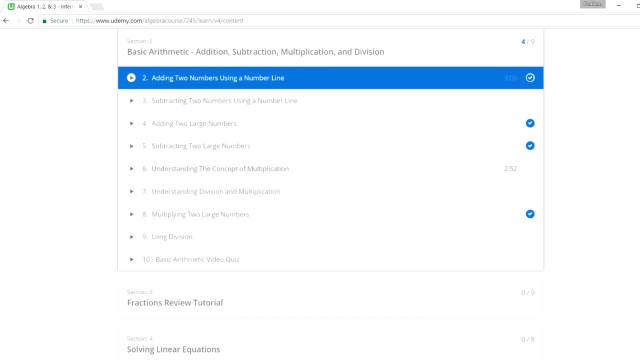 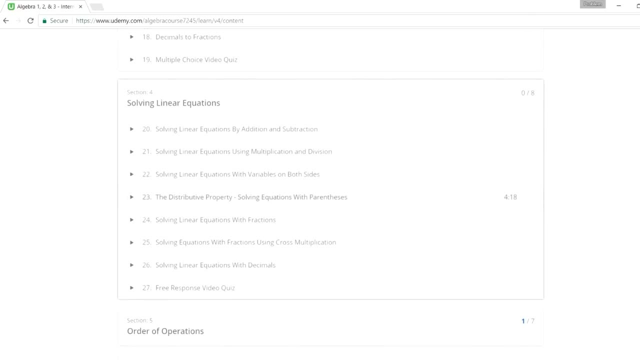 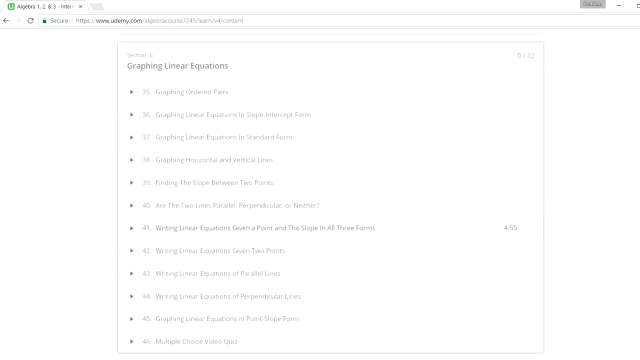 So I have basic arithmetic: addition, subtraction and multiplication. If you want to review a fractions, you can look at section 3. solve a linear solution equations: you have a multiple choice quiz as well. order of operations, graph and linear equations, linear qualities, absolute value, expressions and it's more. 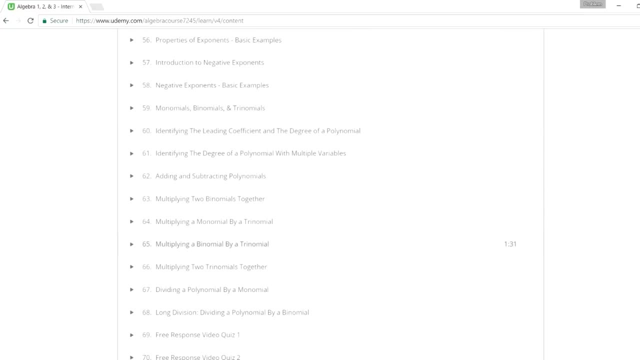 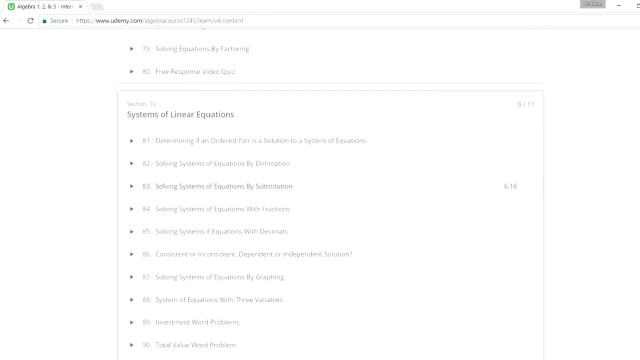 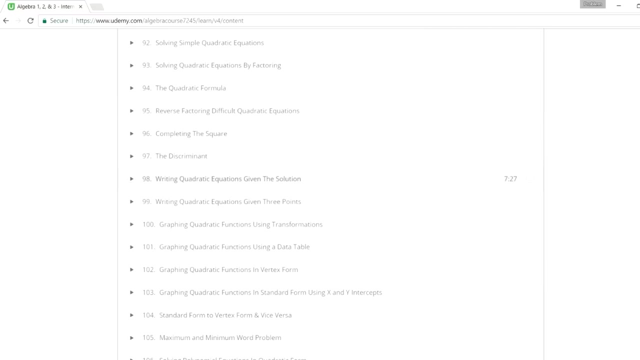 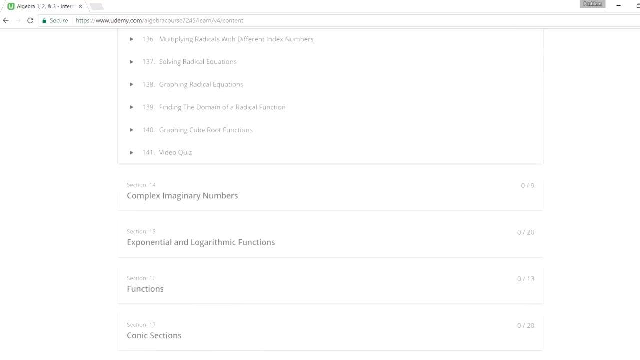 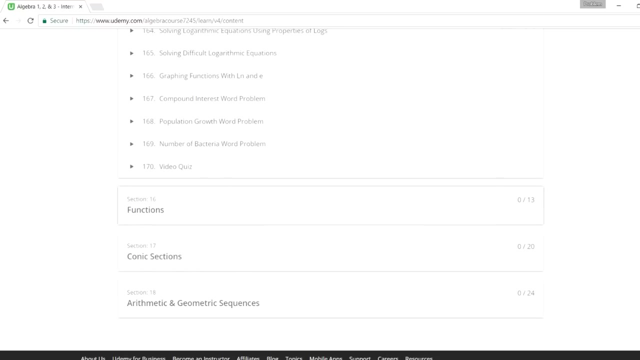 polynomials, multiplying, dividing, things like that, a whole section on factoring, that's a big thing in algebra. and then you have systems of linear equations solving by elimination, substitution, even graphing those things. and then you have quadratic equations, rational expressions, radical expressions and then complex imaginary numbers, exponential functions, logs, how to simplify them. 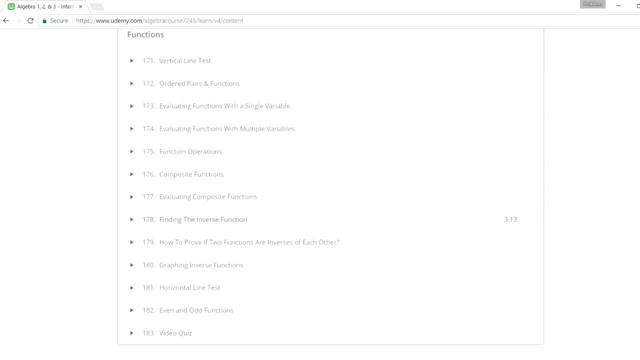 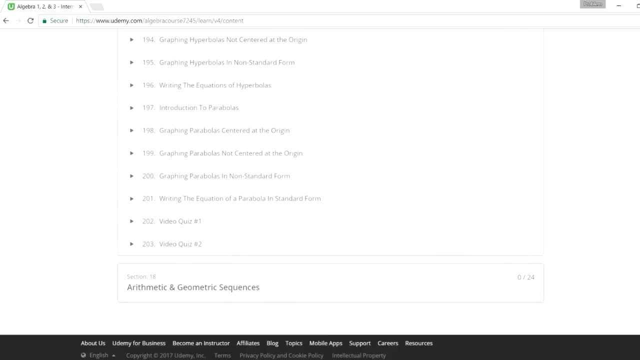 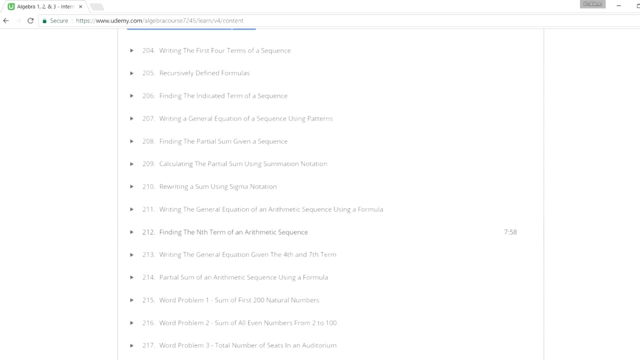 functions in general, like inverse functions, composite functions, and then conic sections, graph and circles, ellipse, parabolas, hyperbolas- There's two video quizzes on that- And finally, arithmetic and geometric sequences. So if you need help in any of these topics, feel free to check out this course when you. 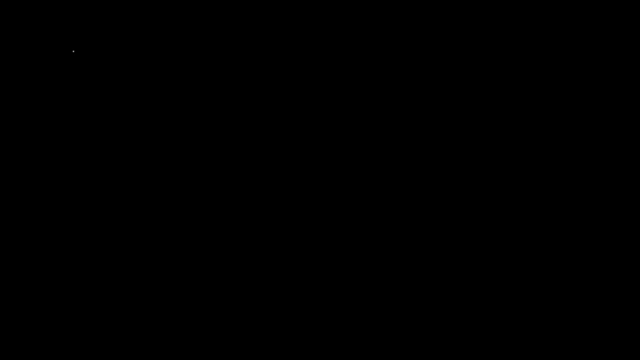 get a chance. Now let's talk about multiplying monomials. What is x squared times x cubed? What is that equal to? When multiplying monomials, you need to add the exponents. Two plus three is five, So it's x to the fifth. 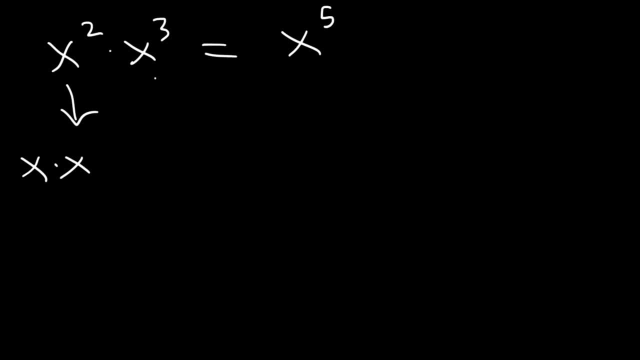 You can see it this way: X squared is x times x, X cubed is x times x times x. So notice that we're multiplying five x variables together, So it's x to the fifth. So try these: X to the fourth times x to the seventh. 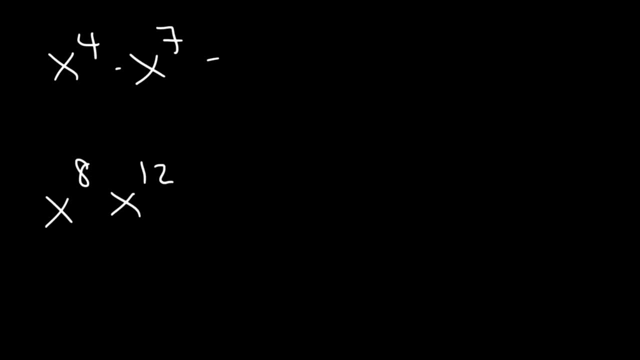 And x to the eighth times x to the twelfth. Go ahead and try those two problems. So this is going to be four plus Plus seven, Which is eleven, And x to the eighth times x to the twelfth, That's going to be x to the eighth plus twelve. 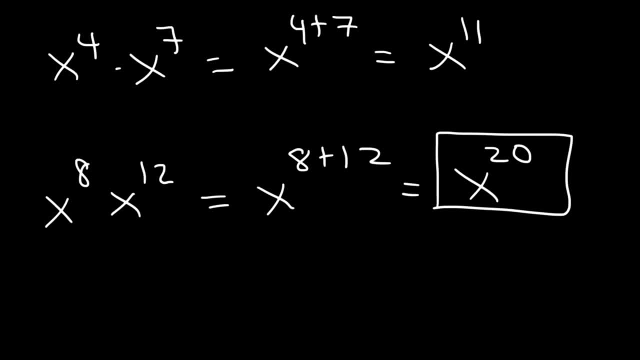 Which is x raised to the twentieth power. So when multiplying monomials you should add similar variables, exponents. Here's another example. Let's say if we have x cubed y to the fifth, multiplied by x to the sixth, y to the eighth, 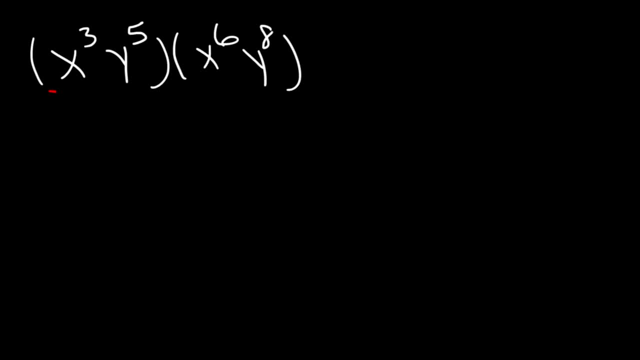 Okay, So first we need to multiply x cubed and x to the sixth, And three plus six is nine, So that's going to be x to the ninth power. And here we have y to the fifth times y to the eighth, So that's going to be y to the thirteenth power. 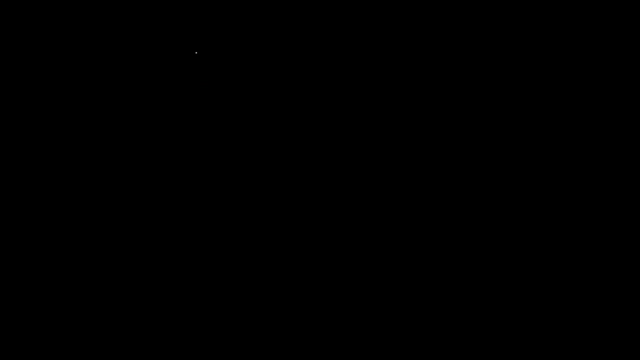 So we have to add all the exponents. Now what about this? one, Three x squared times negative four, x to the fourth power. Go ahead and try that. So first Multiply three and negative four, Which that's going to be negative twelve. 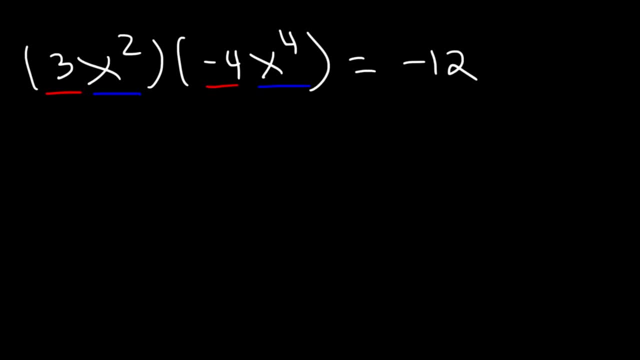 And then we can multiply x squared by x to the fourth, Which is x to the sixth power. So it's negative twelve times x to the sixth. Here's another one: Two x cubed y to the fourth times eight, x to the fifth, y to the seventh. 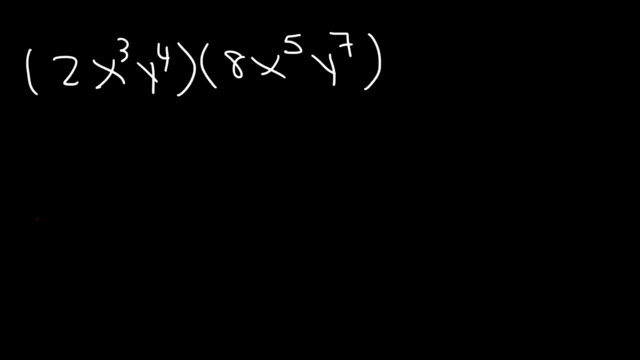 Go ahead and multiply those two terms. So let's begin by multiplying two times eight. Two times eight is sixteen. Next x to the third, times x to the fifth. Three plus five is eight, And then y to the fourth times y to the seventh. 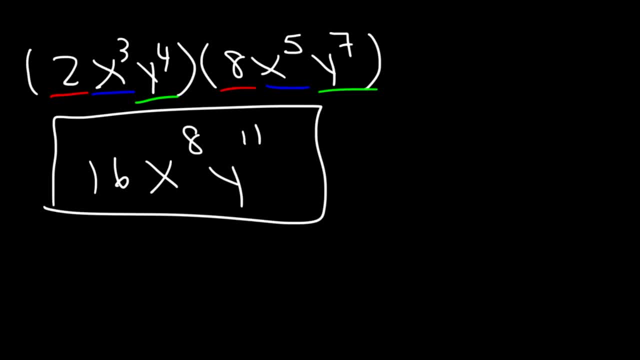 Four plus seven is eleven, And so you should get that answer. Now let's talk about dividing monomials. What is y to the seventh divided by y squared? Okay, When multiplying you should add the exponents, But when dividing you need to subtract the exponents. 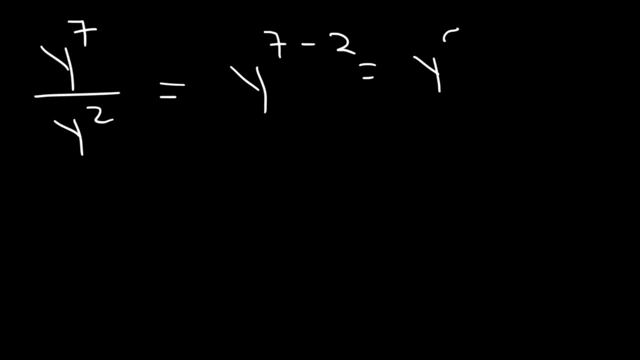 So this is going to be seven minus two, Which is five. Now to explain it, let's use factorization. Y to the seventh means that we have seven y variables multiplied together. Y squared is just y times y. We could cancel two of them. 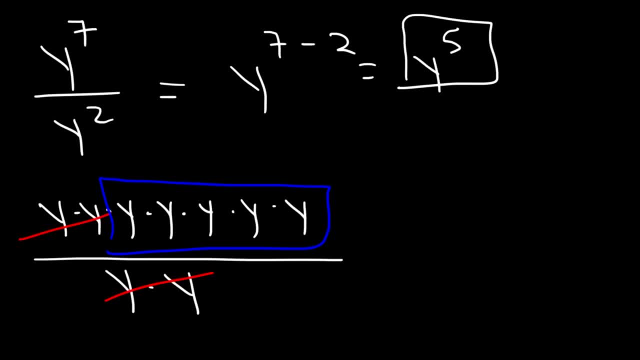 But notice that we have five y variables left over. So that's why it's simply y to the fifth over one Which is y to the fifth. Now, what is three to the seventh divided by three to the third power? Go ahead and try that. 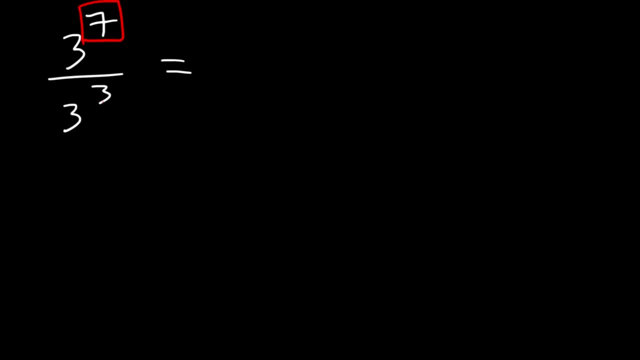 So we know that we need to subtract the exponents. Seven minus three is fourth, So this is three to the fourth power, Which is three times three times three. Three times three is nine, So we have nine times nine, which is eighty-one. 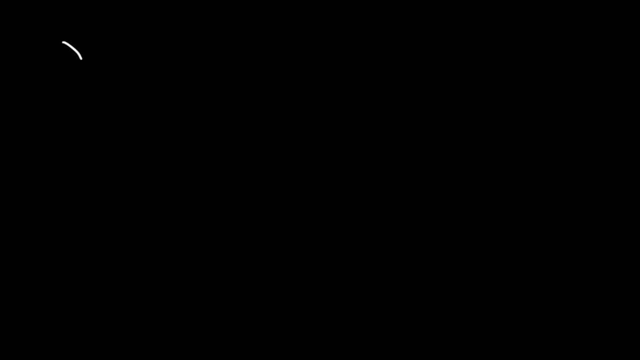 And so that's the answer for this example. Now, what is x cubed times x to the eighth, divided by x to the fifth power? So to begin, in order to simplify this expression, let's multiply x cubed by x to the eighth. 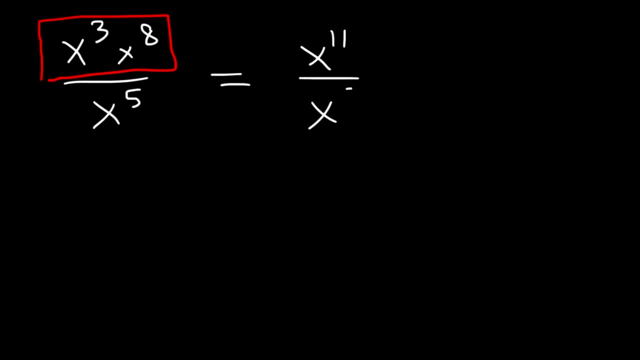 first: Three plus eight is eleven. Now, at this point, we could divide: Eleven minus five is six, And so that's going to be the final answer. Here's another one that you could try: Y to the eighth, divided by y, squared times, y cubed. 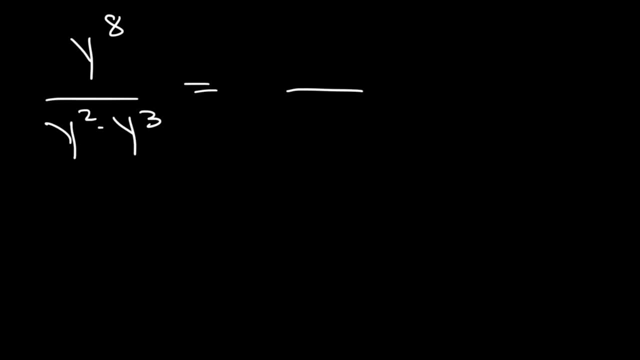 So take a minute and work on that example. So first I would multiply the two on the bottom, which I think is easiest to do first. Two plus three is five. And now it's best to divide: Eight minus five is three. 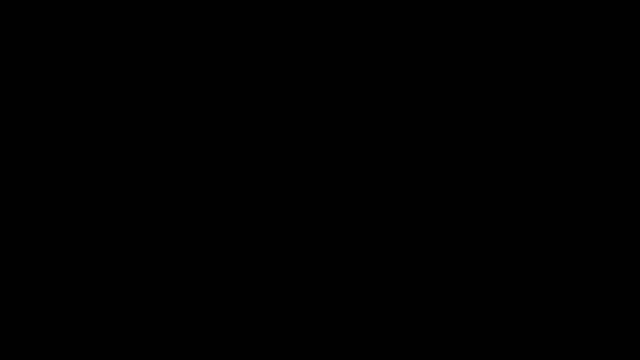 So the answer is y to the third. Now try this one. What is x squared divided by x? to the seventh? That's going to be two minus seven. You take the top number first and subtract it by the one on the bottom. Now this is equal to x to the negative five. 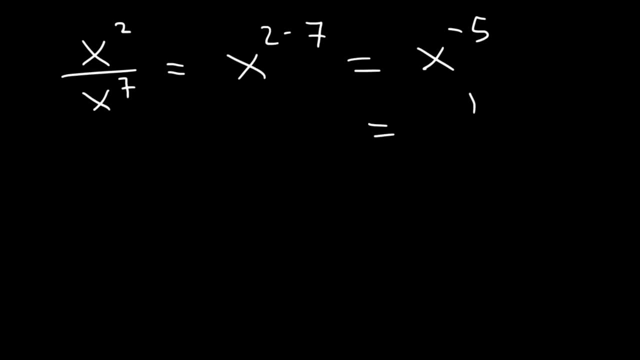 So what does that mean? X to the negative, five is one over x to the five. So when you have a negative exponent, what you need to do is move the variable to the bottom and the negative exponent will change, sign It's going to become positive. 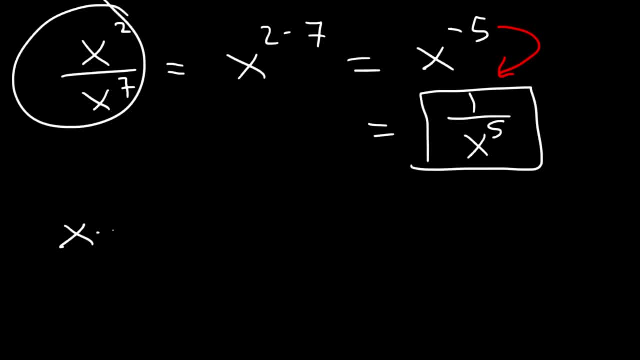 To verify. we could simplify this another way: X squared is x times x And x to the seven. we know it's basically seven x variables multiplied to each other, two of which can be cancelled. So we have five x variables on the bottom. 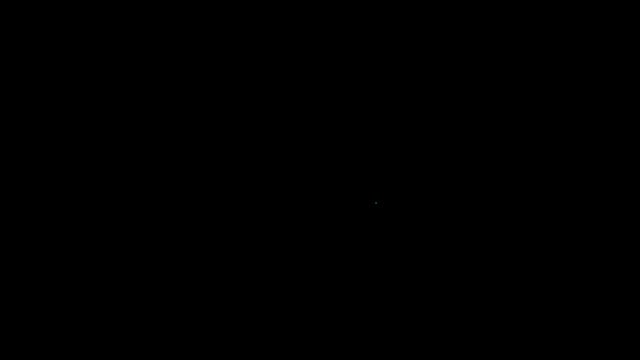 Thus it's one over x to the fifth power. Subtitles by the Amaraorg community. So what is three to the negative one power? So right now the three is on the numerator of the fraction. If you bring it to the denominator it's going to have a positive one exponent. 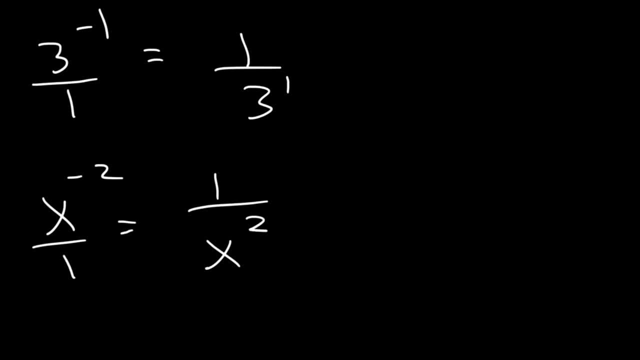 X to the negative. two is equivalent to one over x squared And one over x to the negative. four is x to the positive four. So when you move a variable or a number from the top to the bottom or to the bottom, you're going to have a negative one exponent. 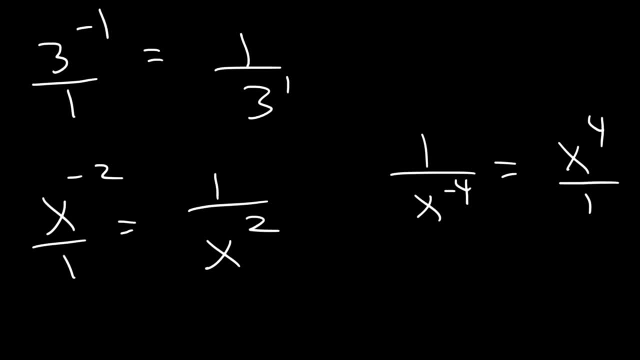 And the exponent changes sign. It can switch from negative to positive. What is negative? four raised to the negative? two power. So first we need to bring it down. This is negative. four raised to the second power: Negative four squared is positive sixteen. 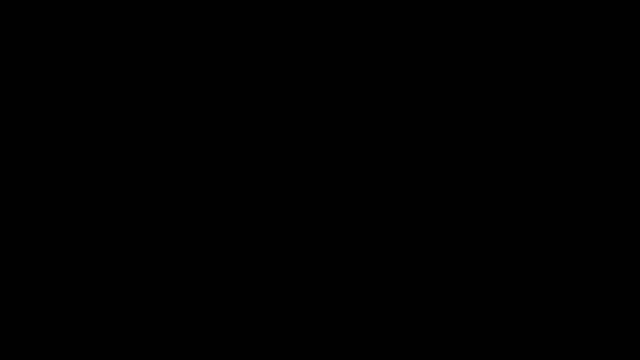 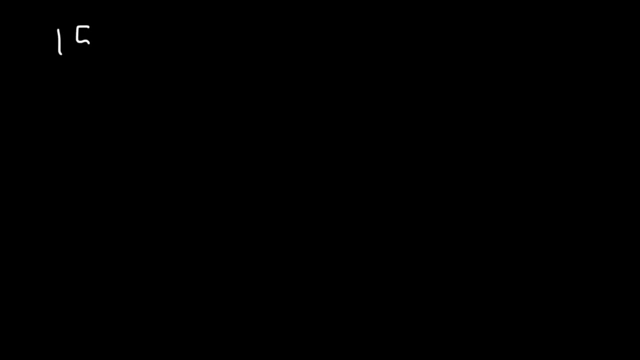 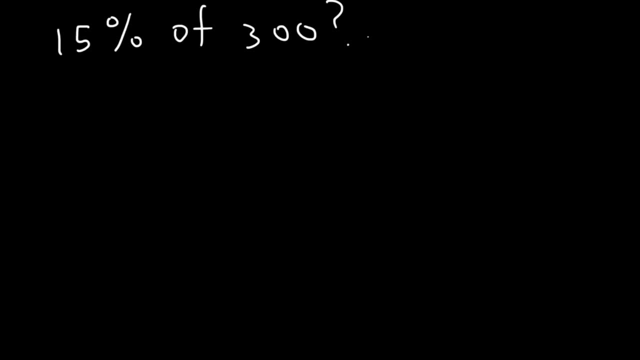 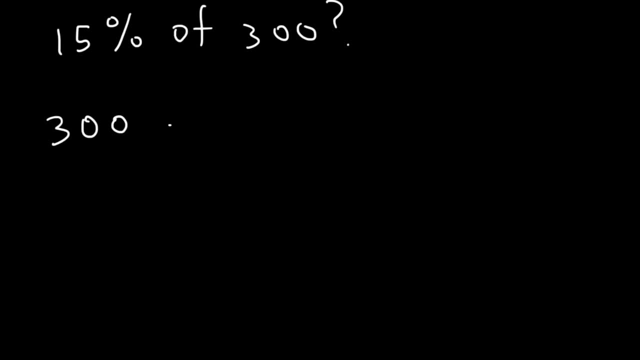 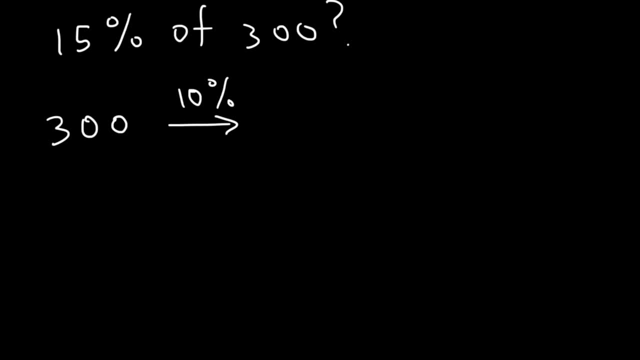 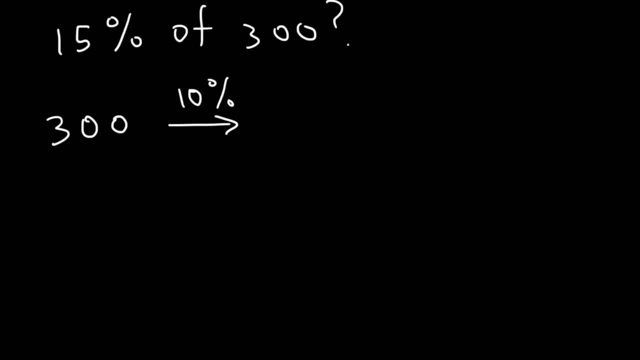 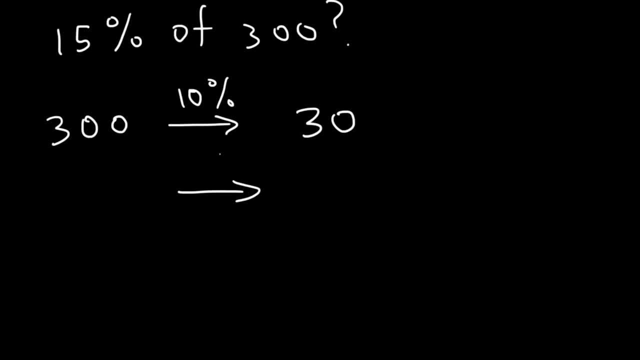 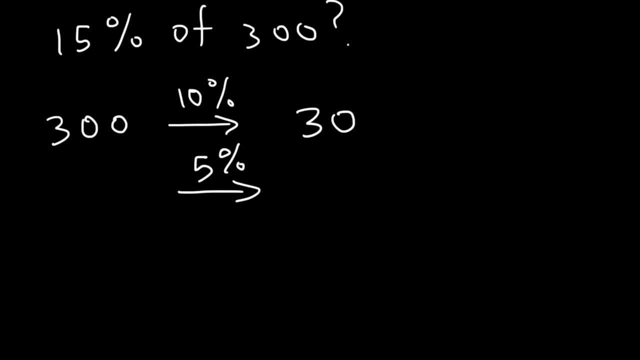 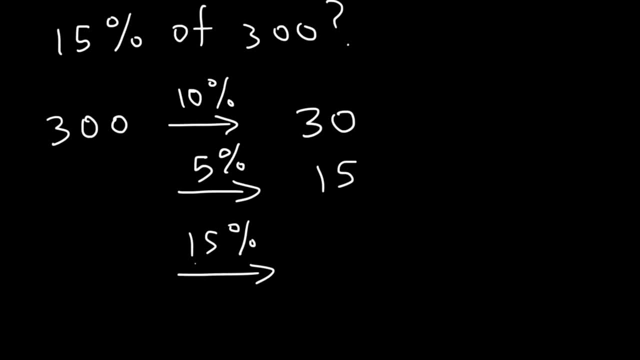 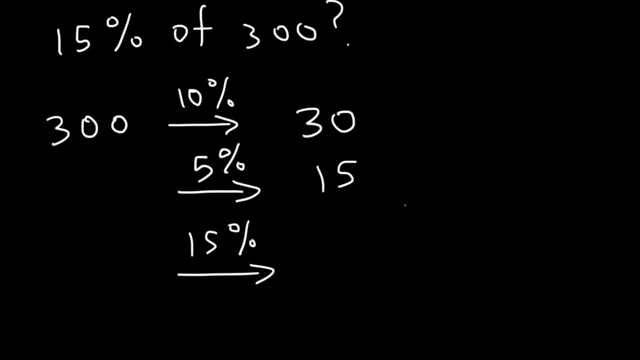 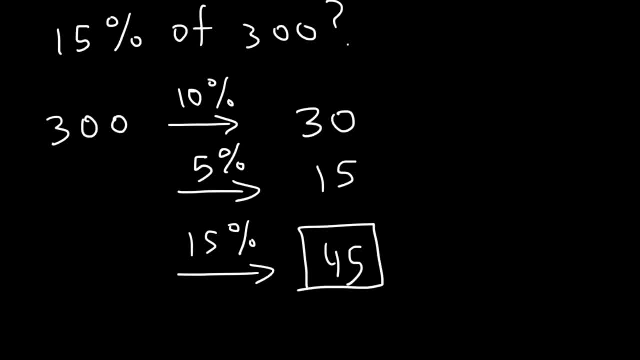 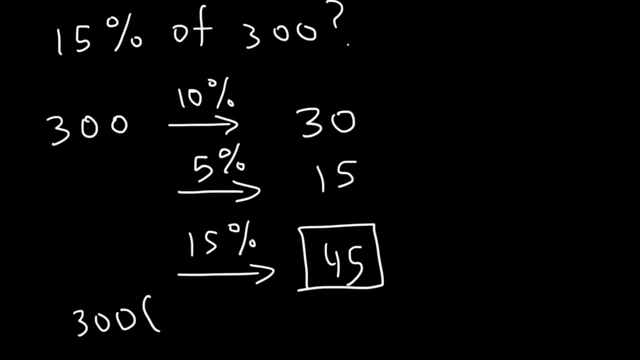 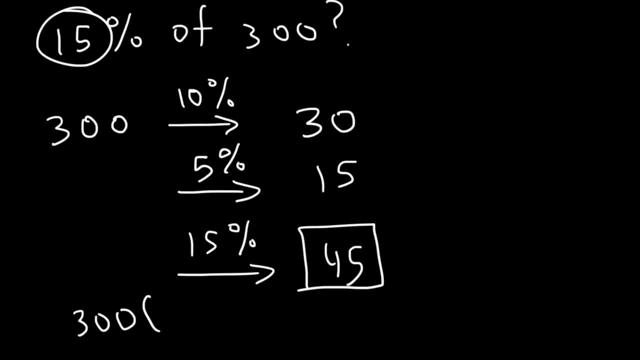 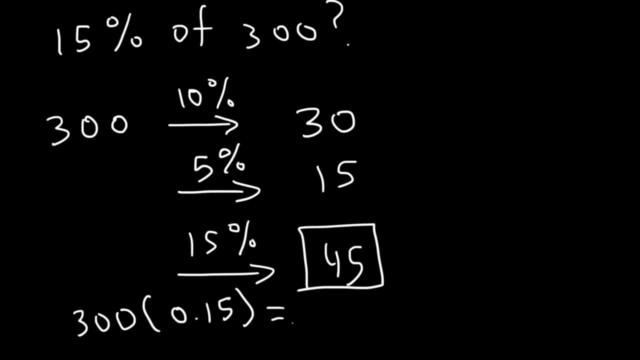 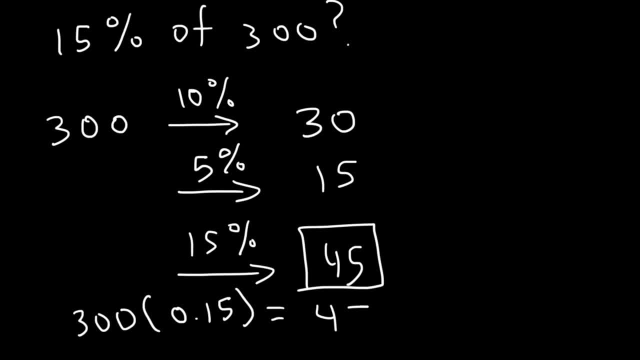 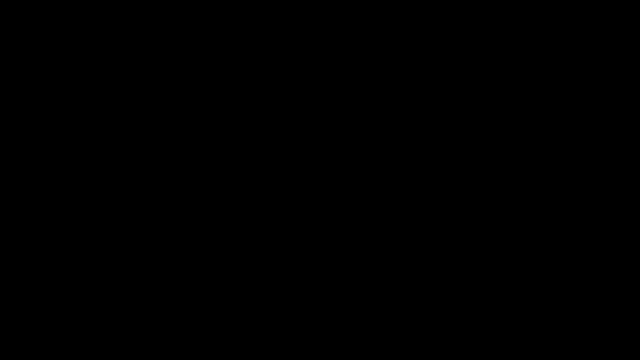 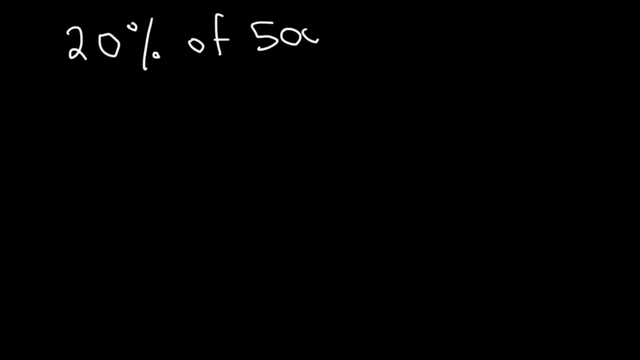 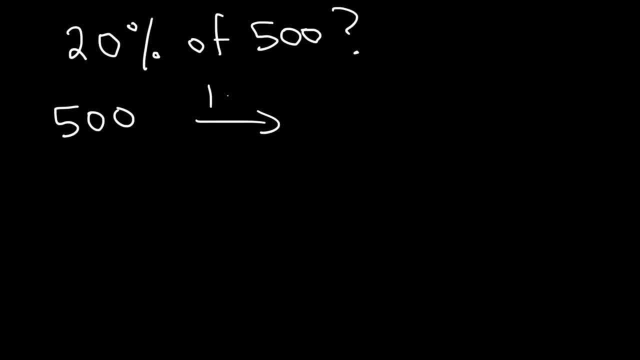 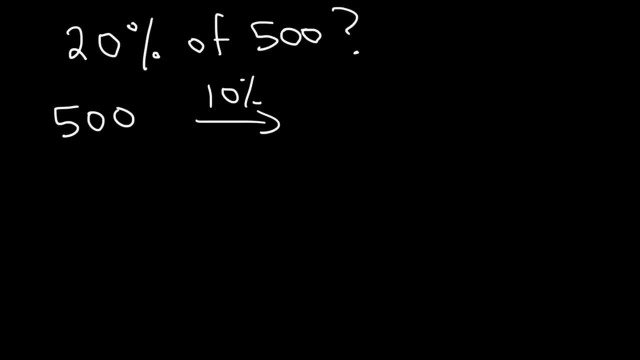 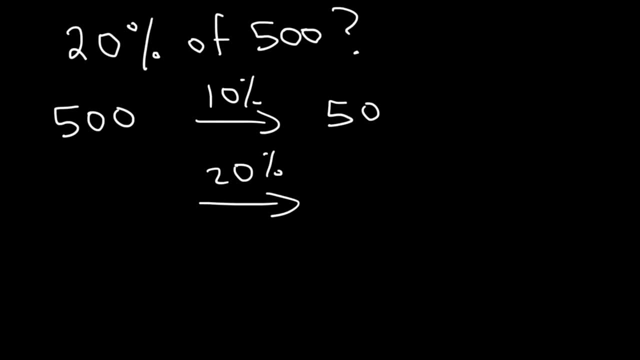 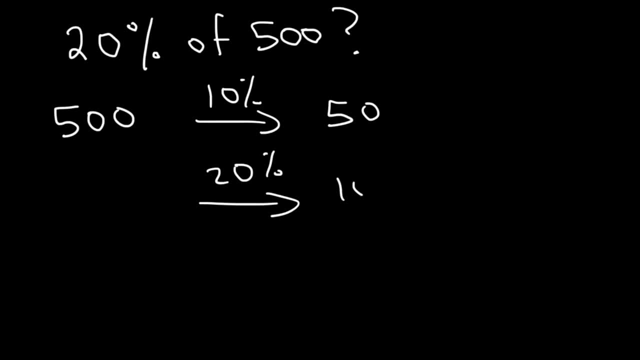 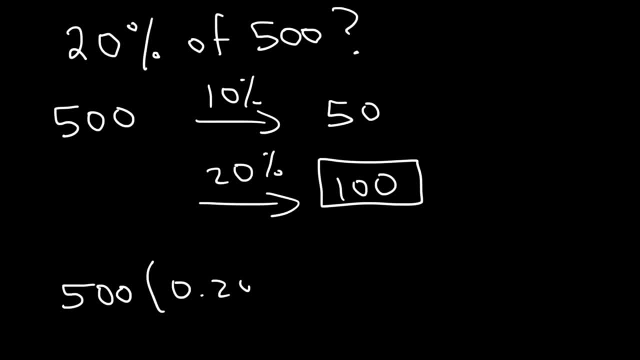 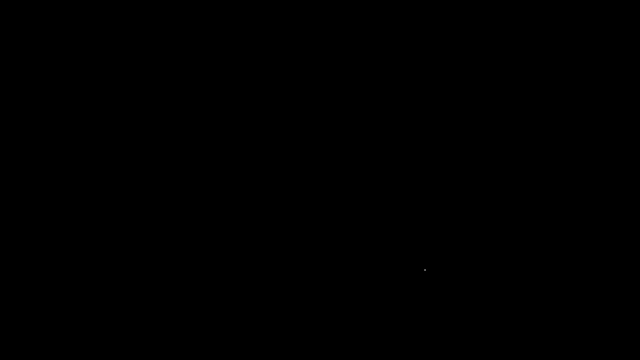 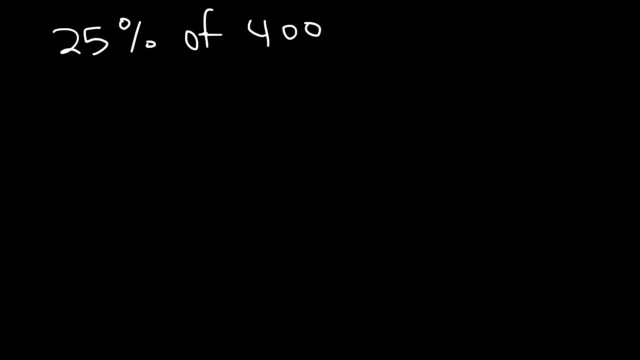 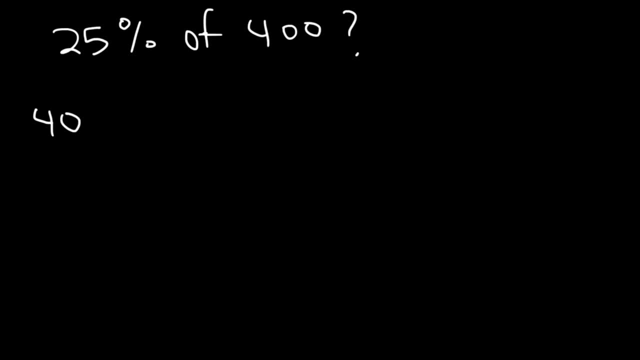 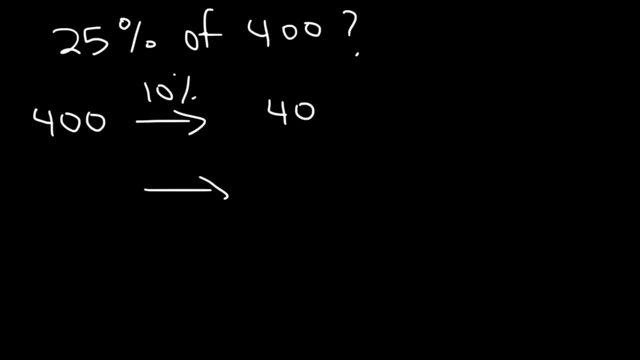 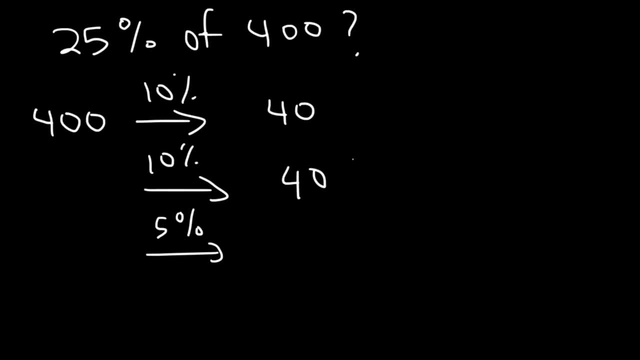 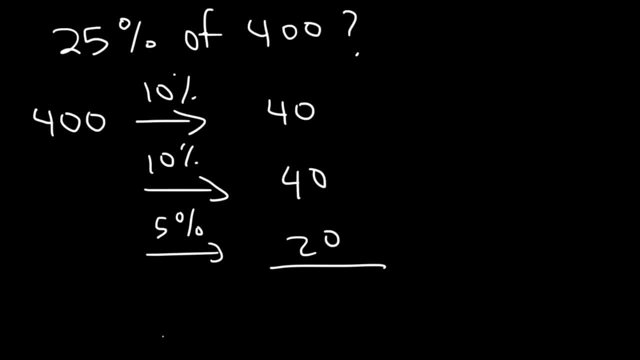 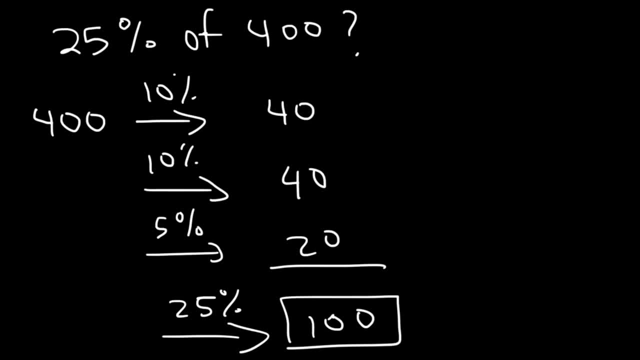 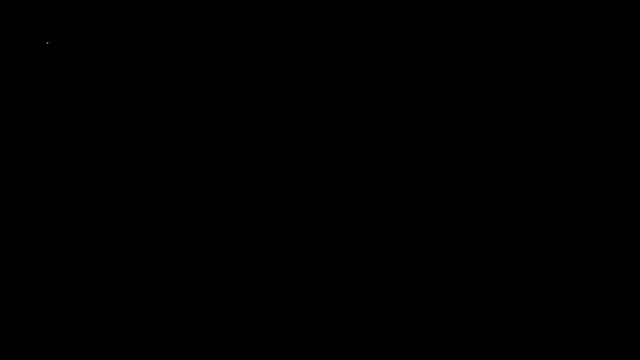 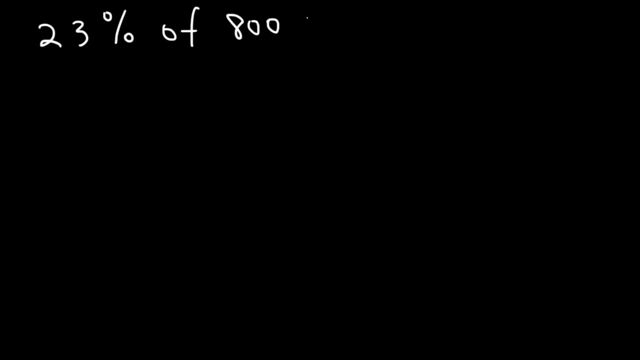 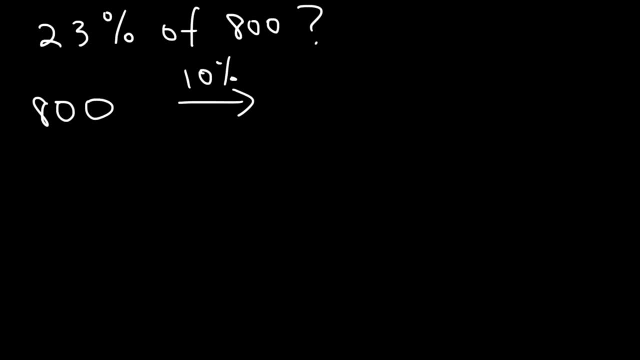 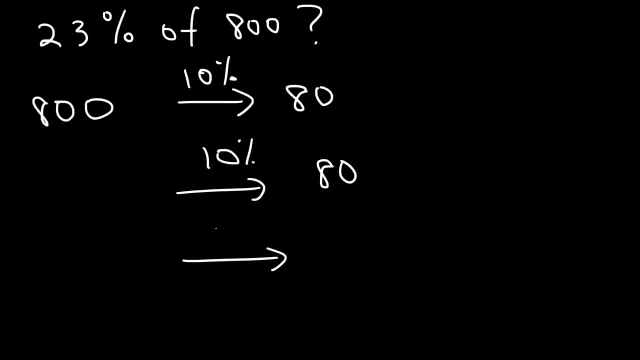 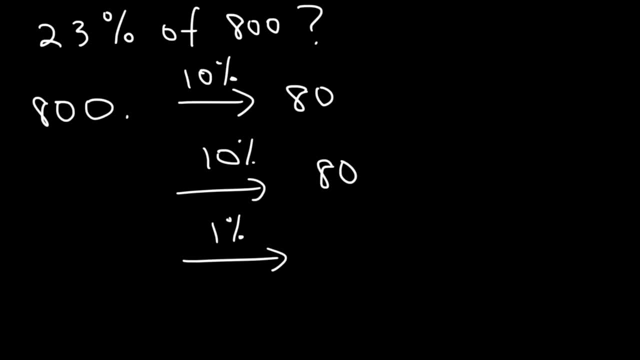 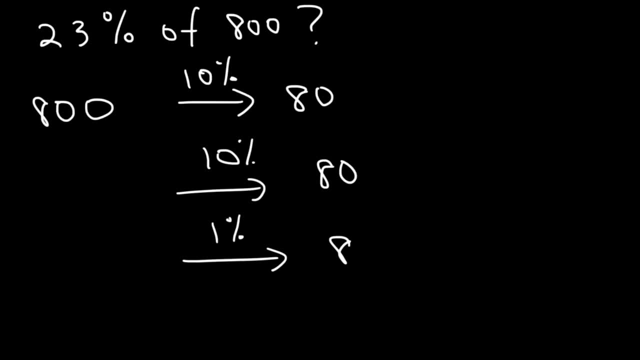 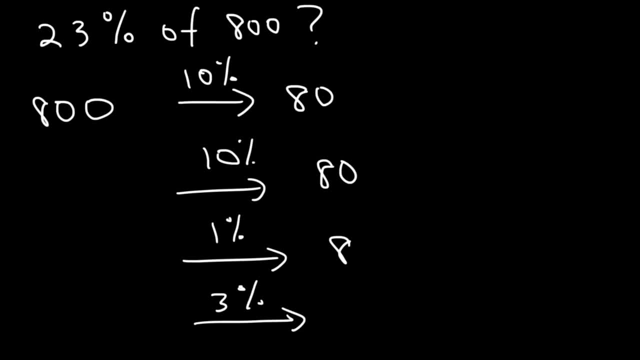 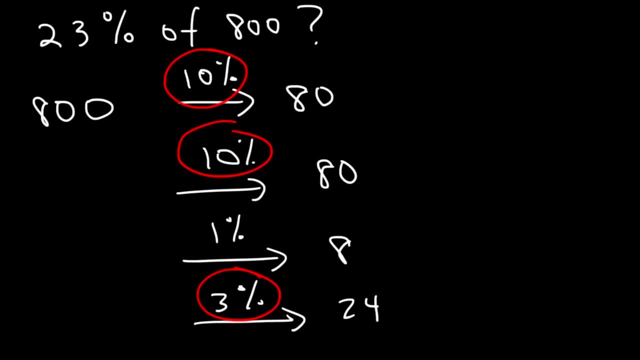 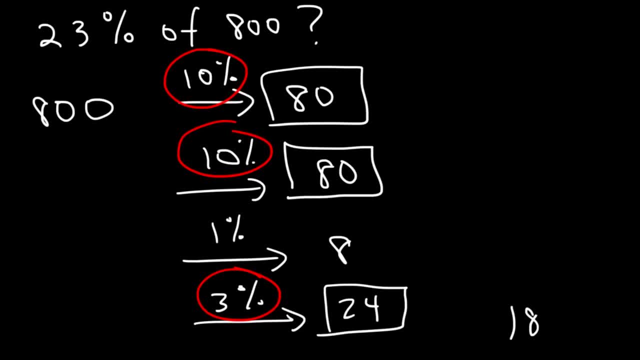 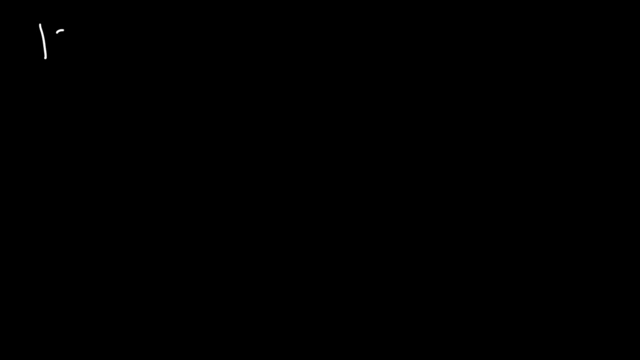 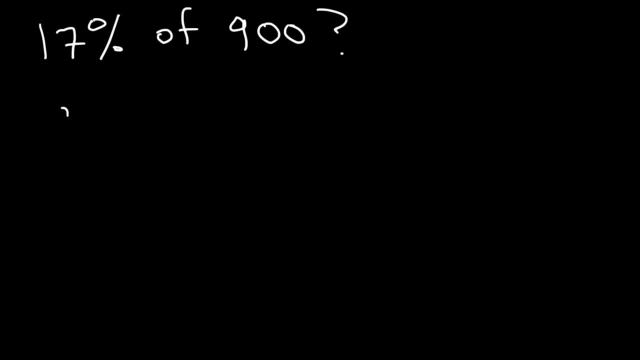 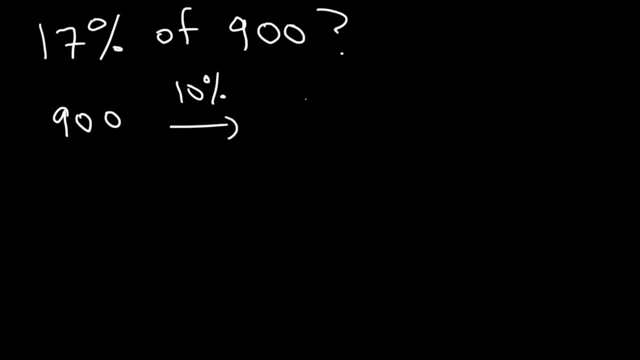 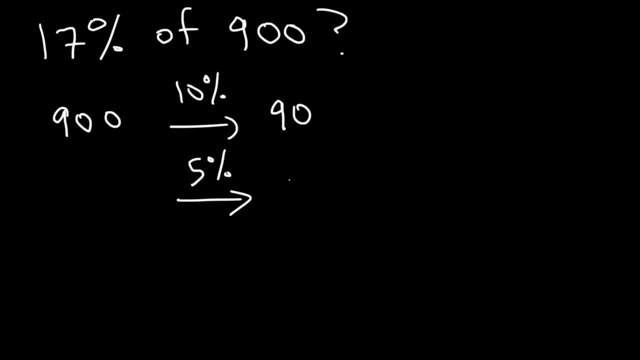 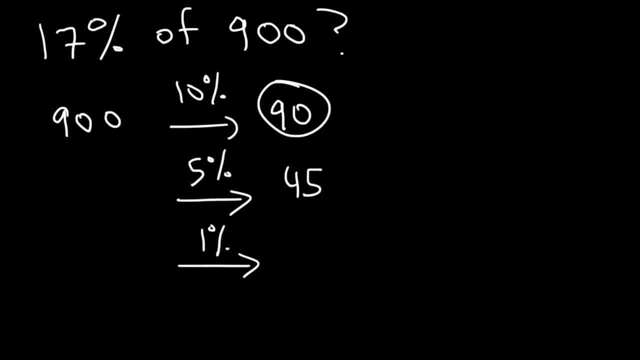 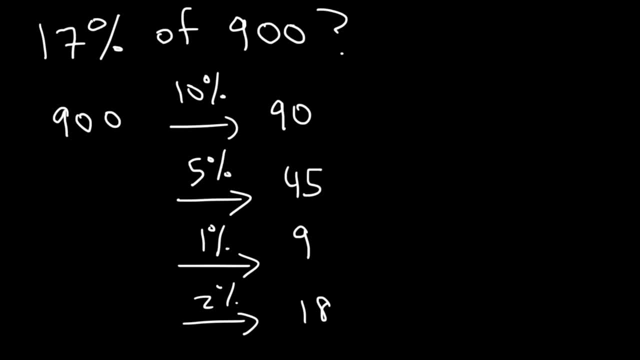 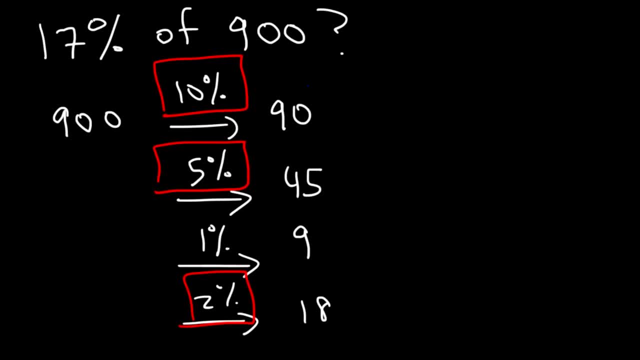 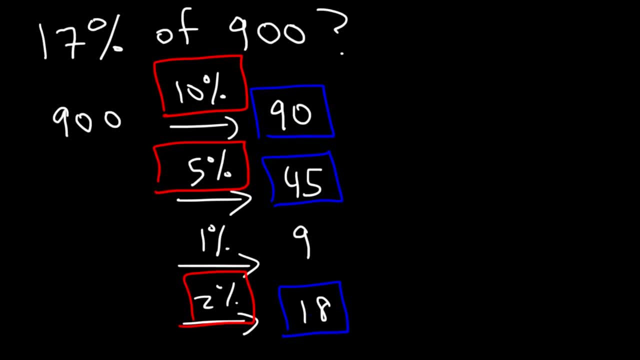 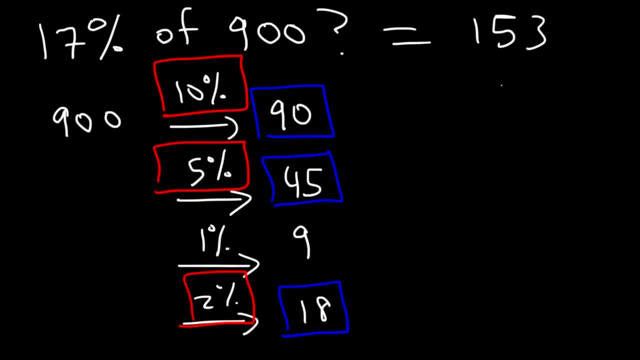 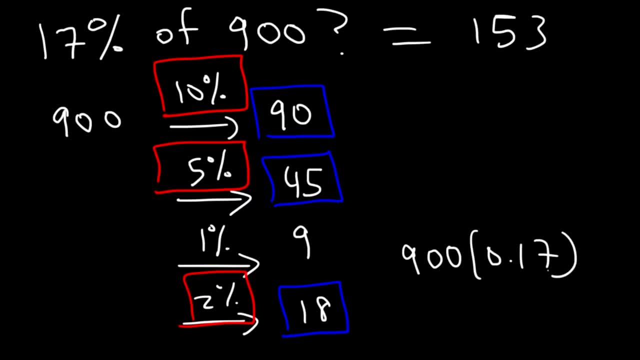 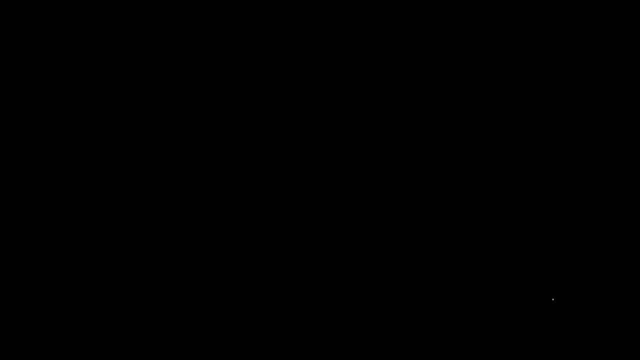 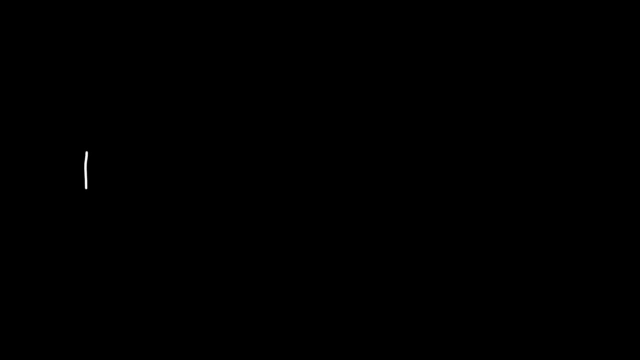 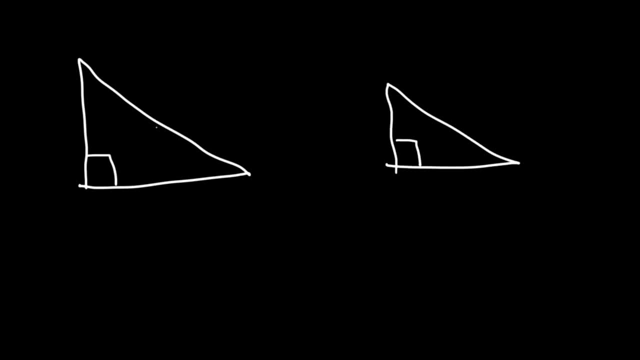 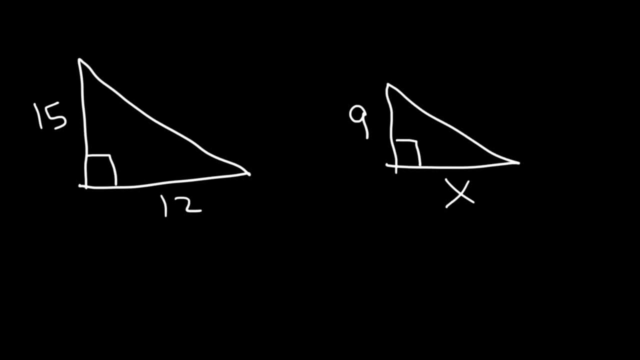 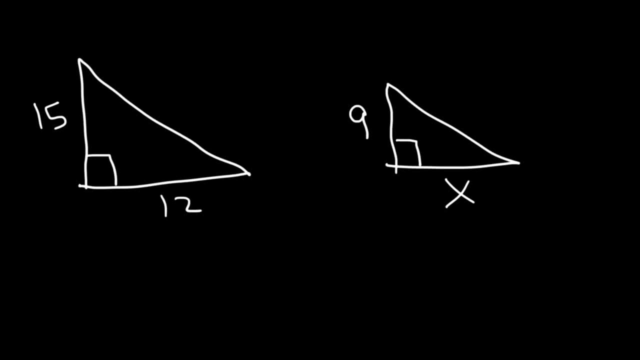 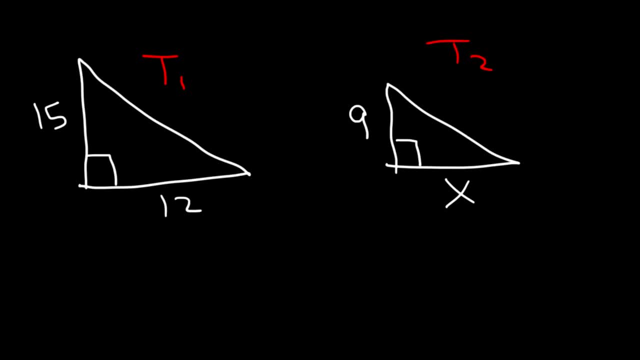 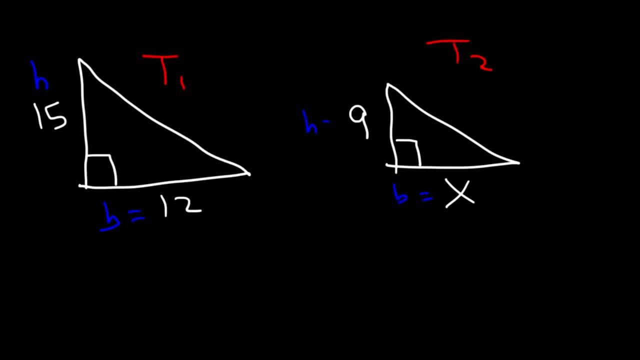 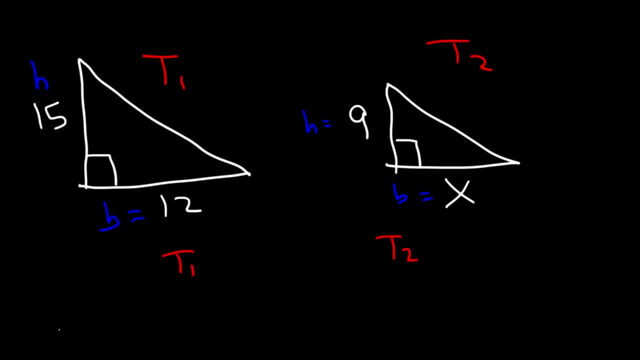 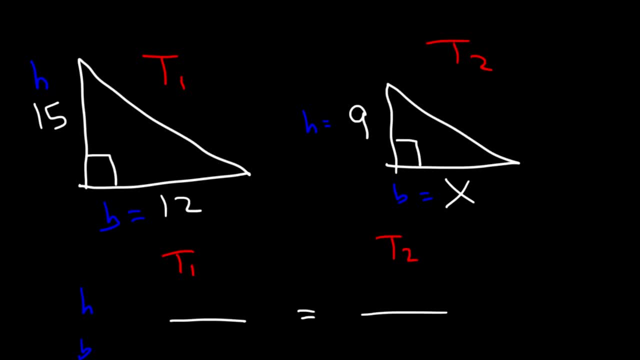 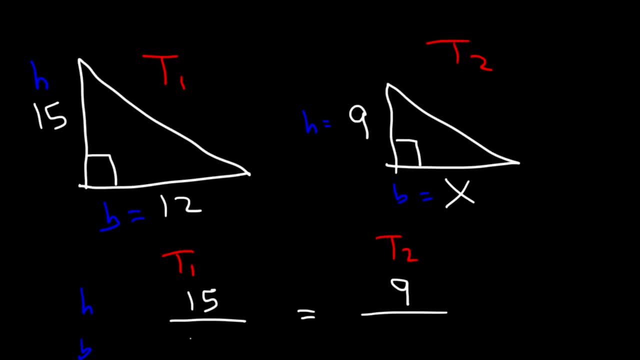 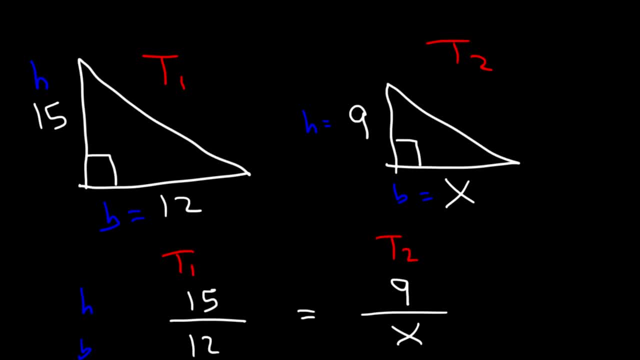 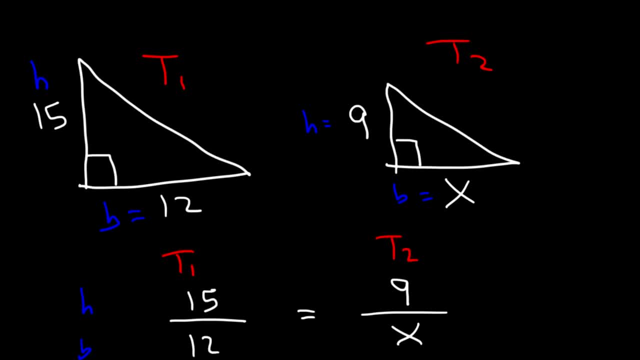 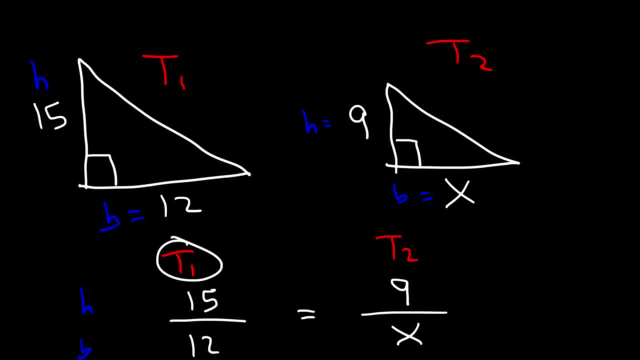 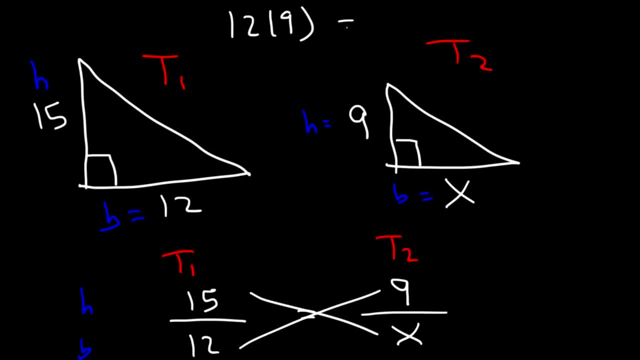 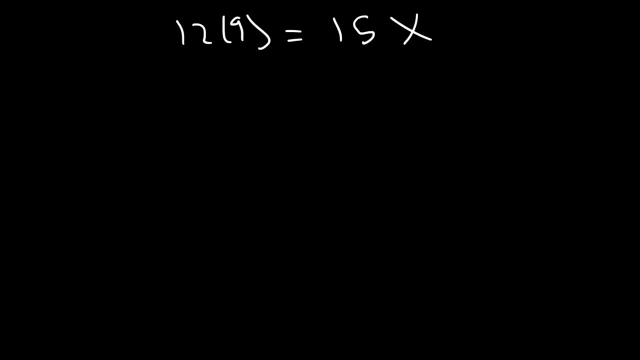 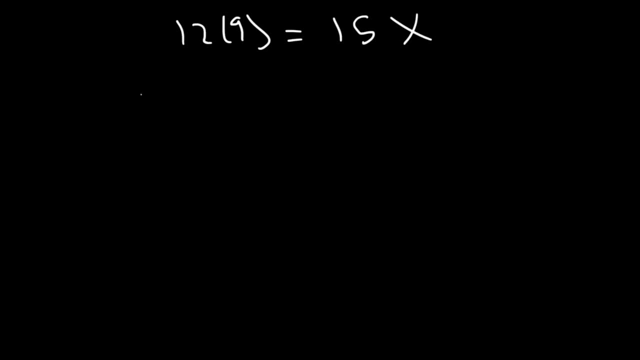 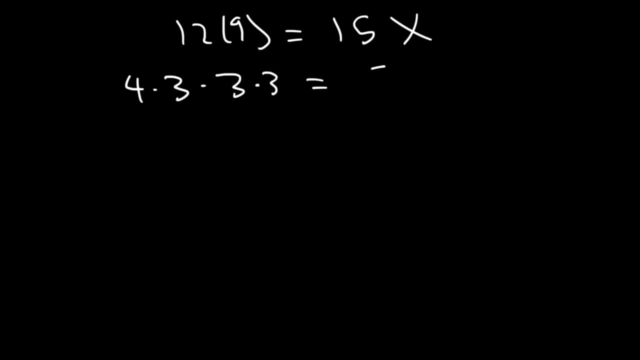 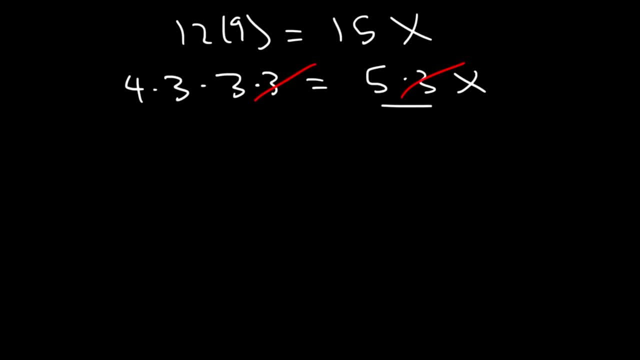 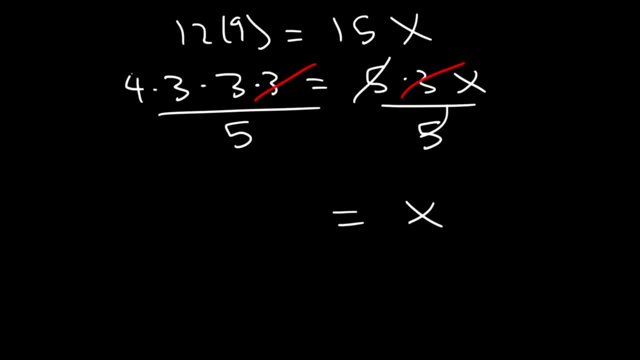 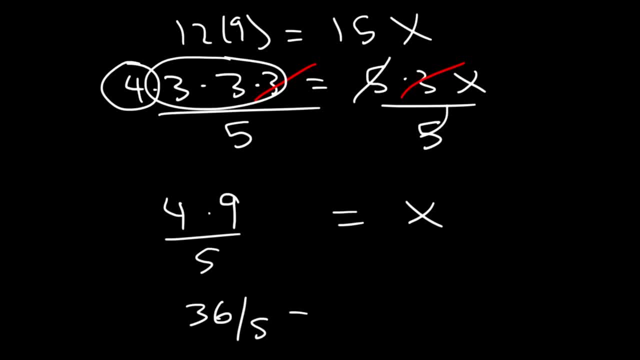 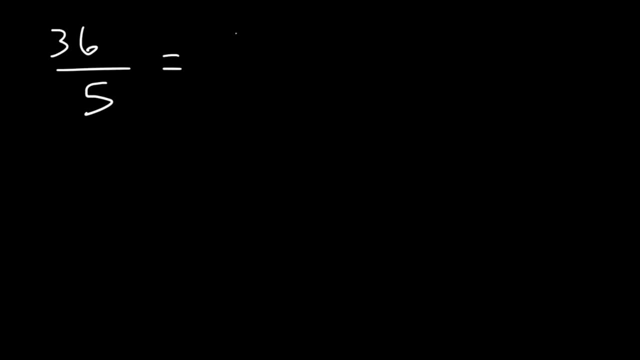 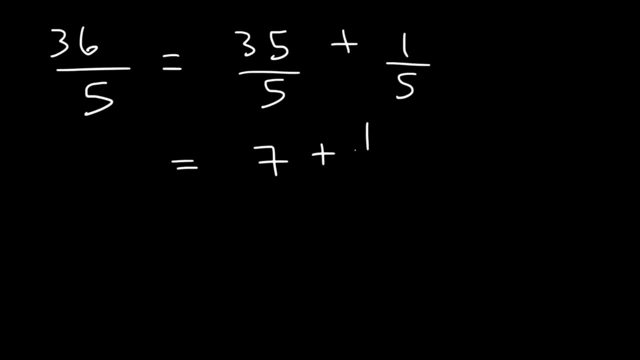 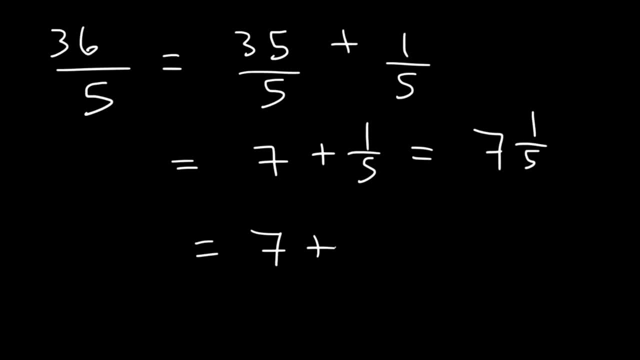